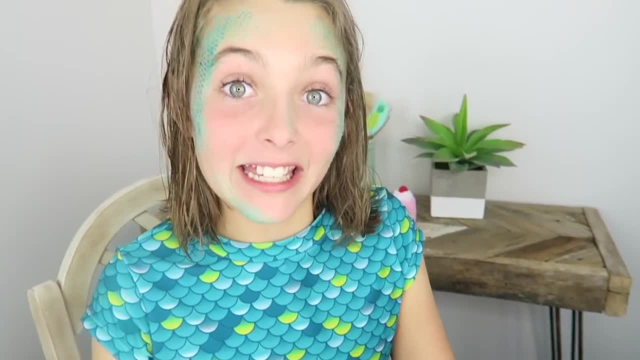 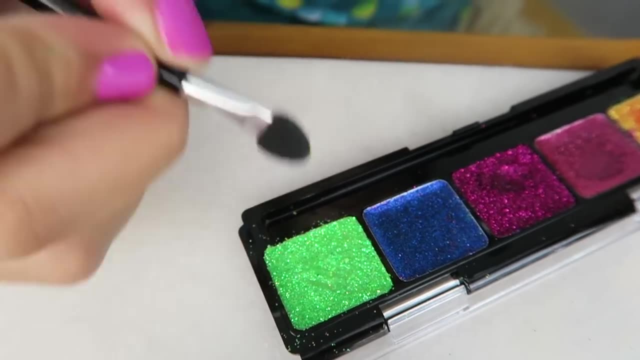 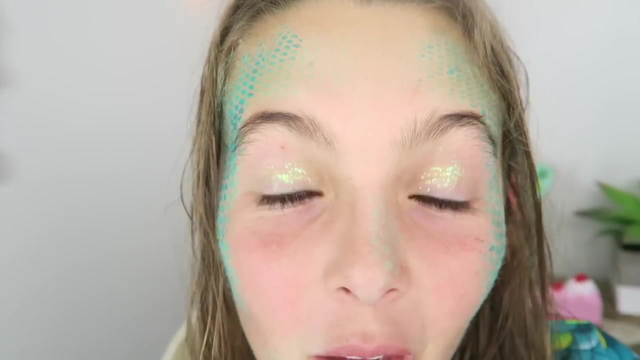 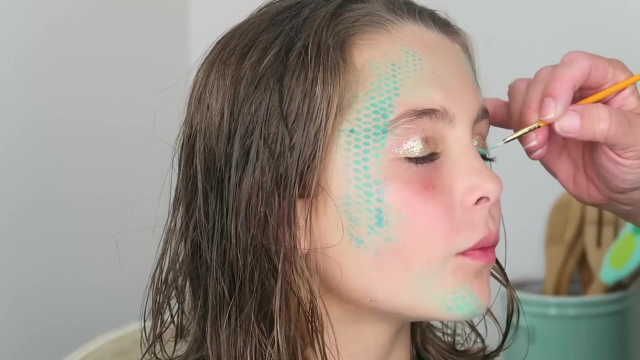 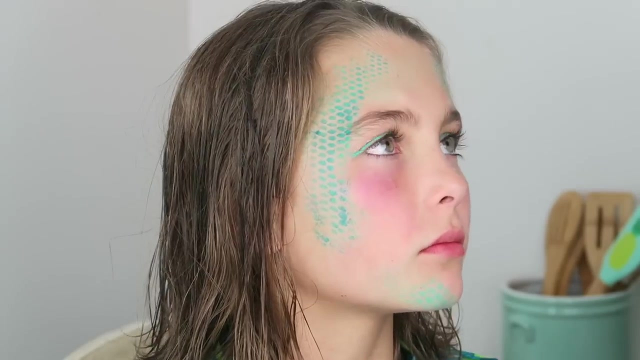 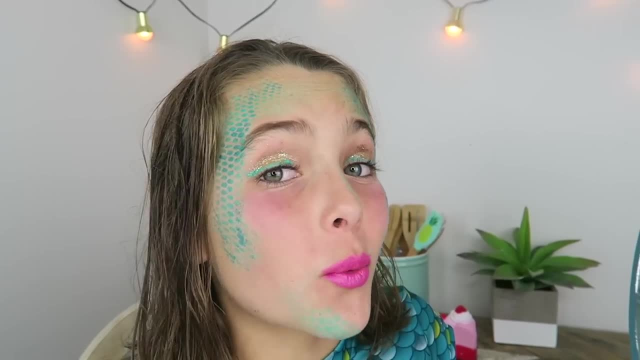 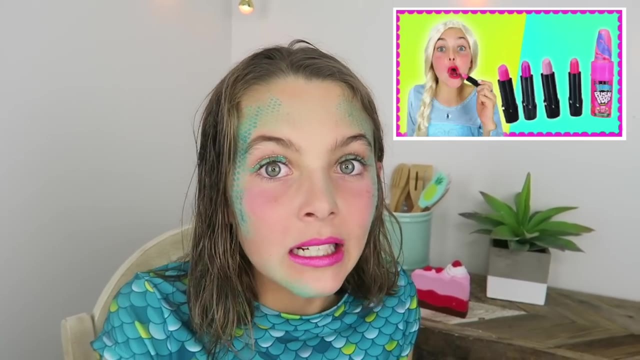 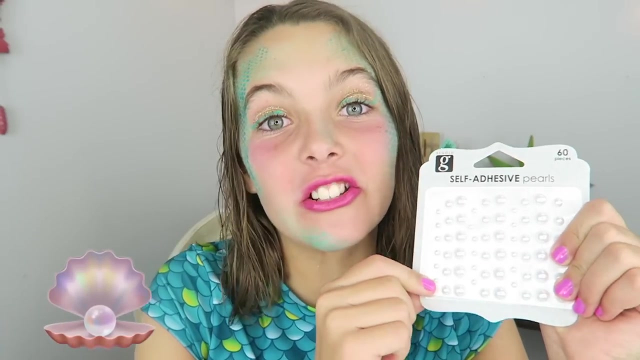 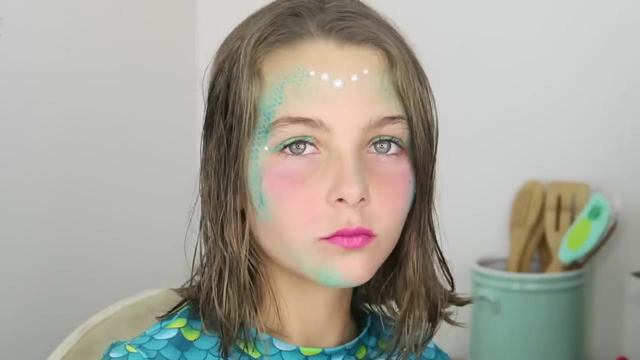 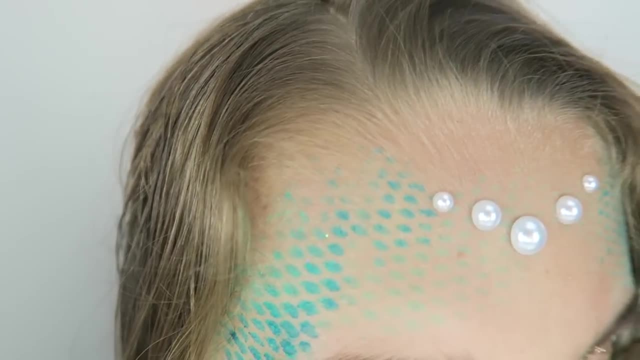 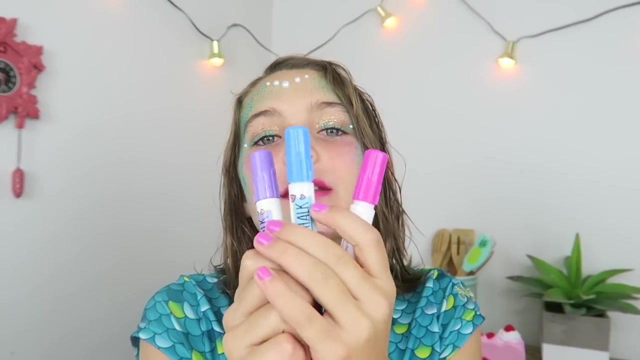 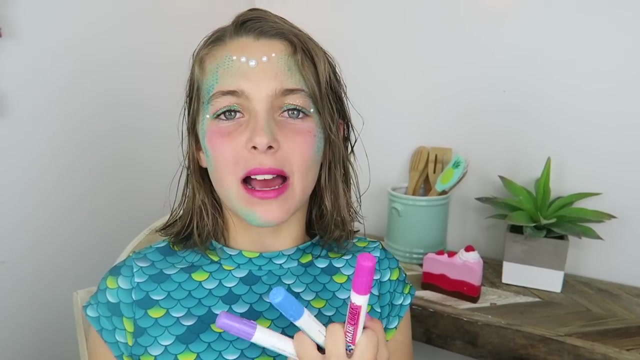 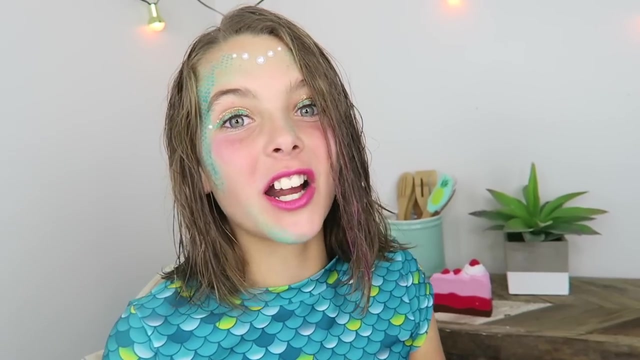 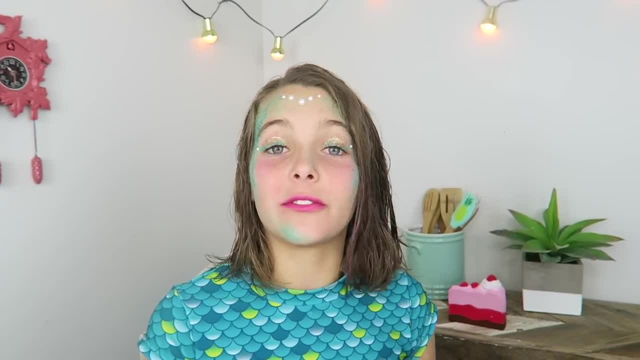 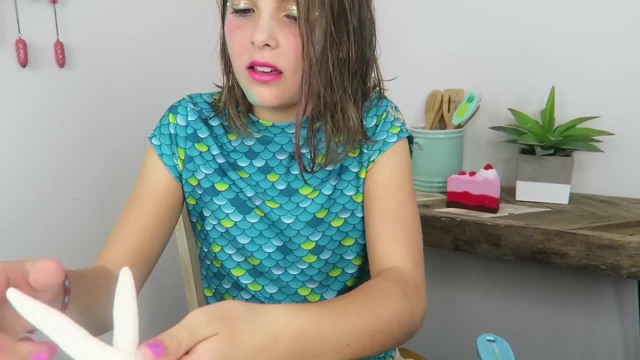 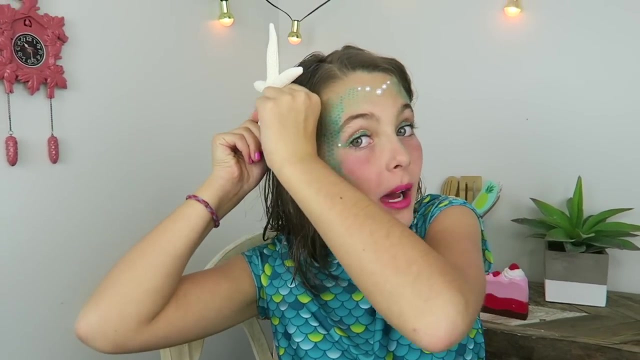 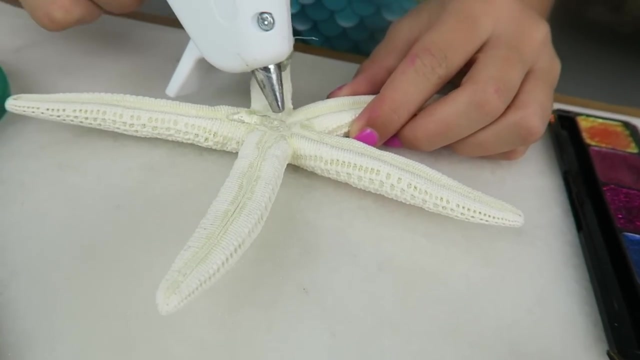 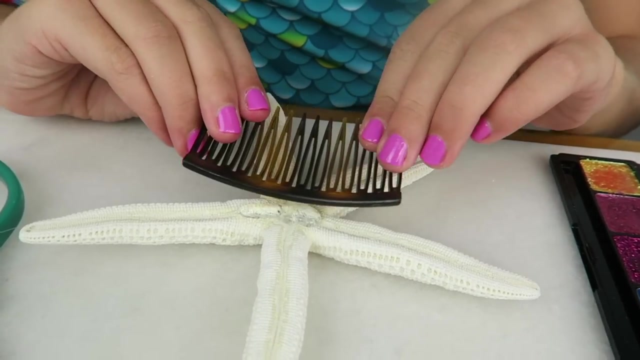 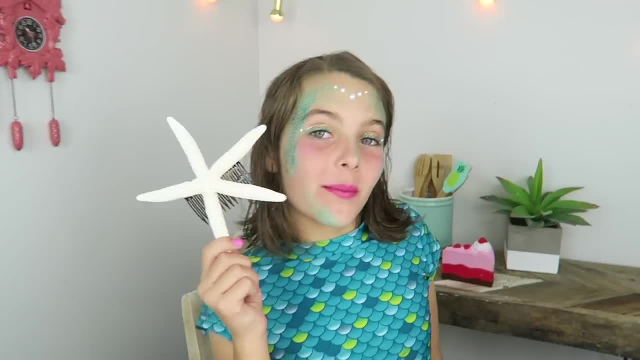 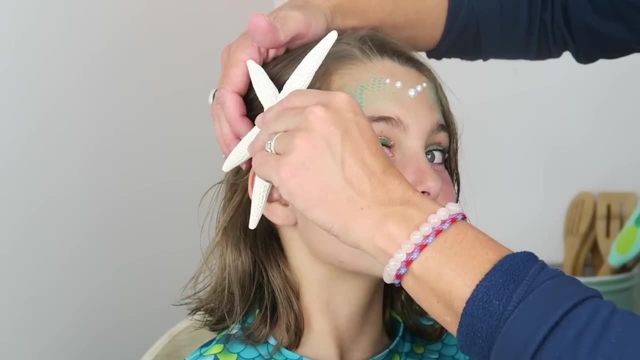 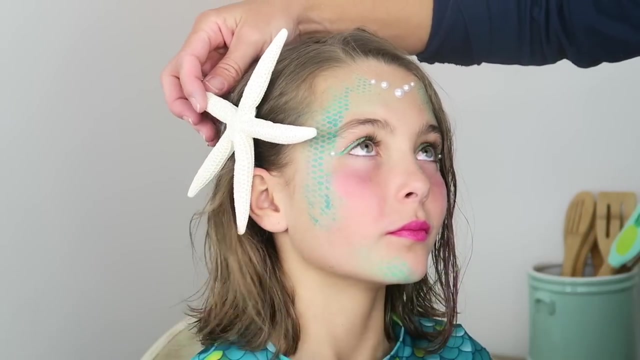 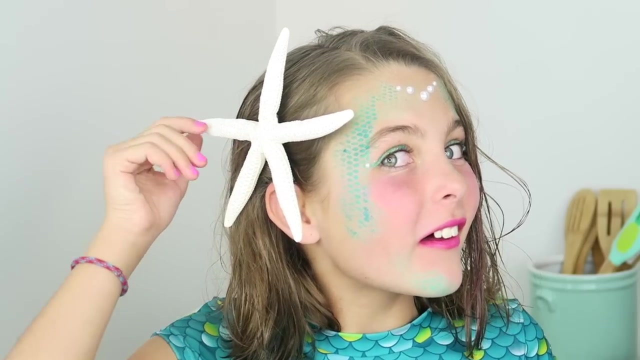 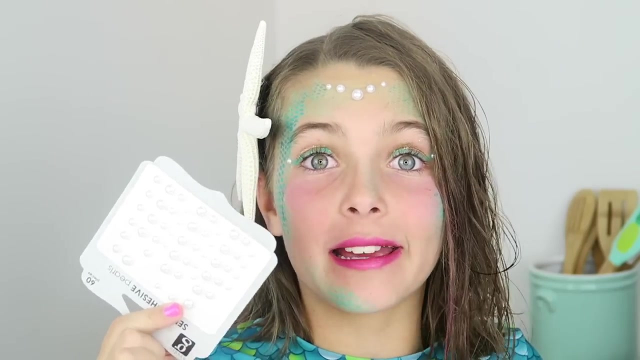 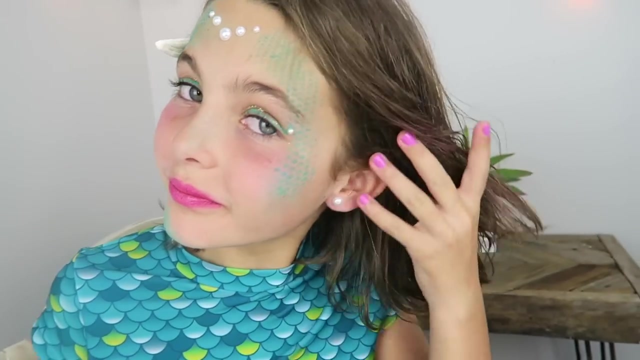 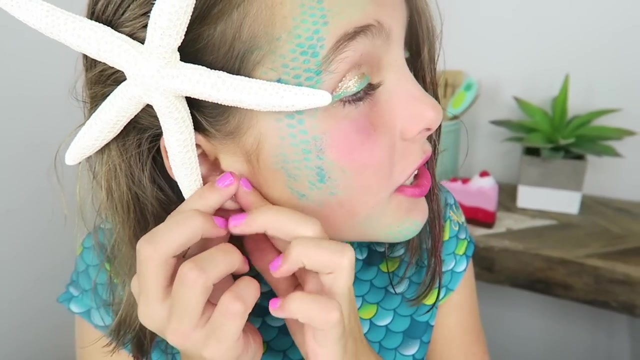 that now you have a mermaid hair accessory. whoa, guys, isn't this so cool. okay, time for the earrings. so the pearls that we use for our head, we're gonna use it as earrings, so I'm just gonna grab the biggest pearls. hey, I got it on straight. my ears are actually Pierce. it's just, this is a lot. 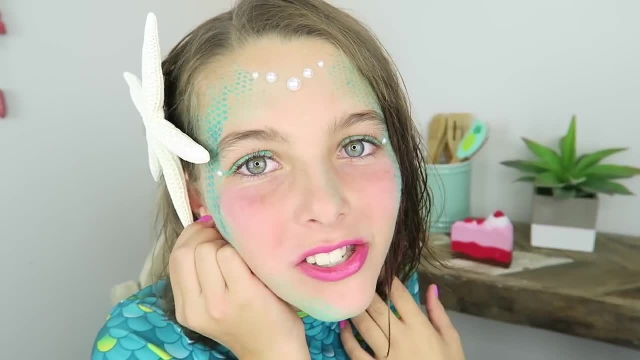 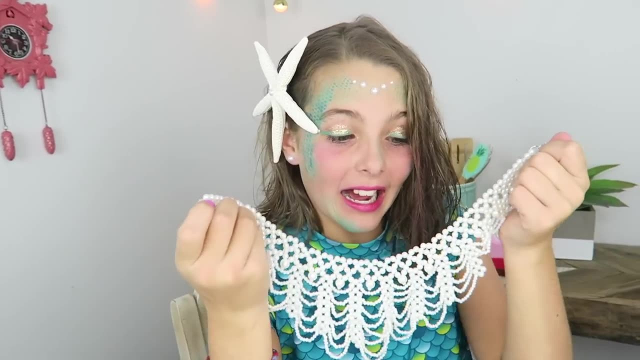 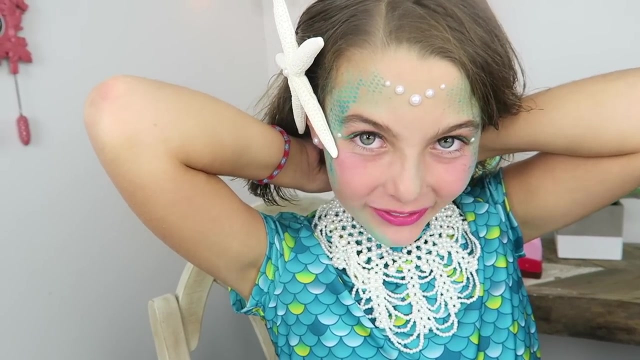 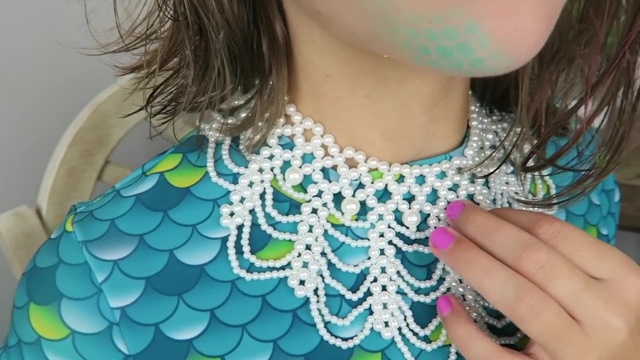 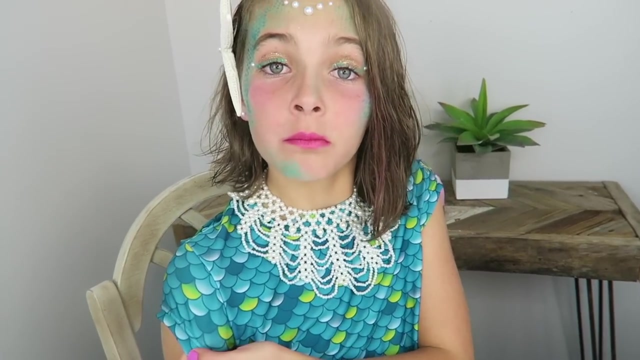 easier. comment down below if your ears are pierced there. time for the finishing touch. look at this amazing necklace that I got. I actually borrowed it from my mom. okay, just gonna. lots of pearls going on here. voila, this is actually my swimsuit. I'm ready for my Halloween party, are you guys? 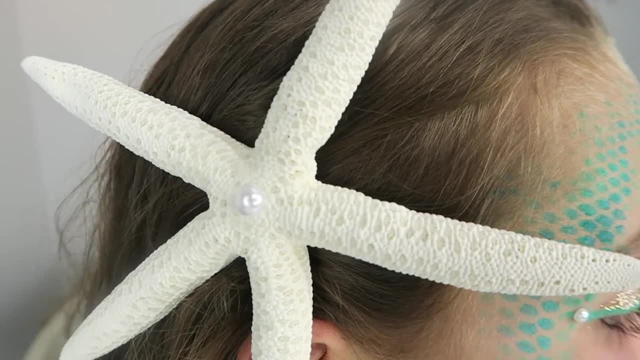 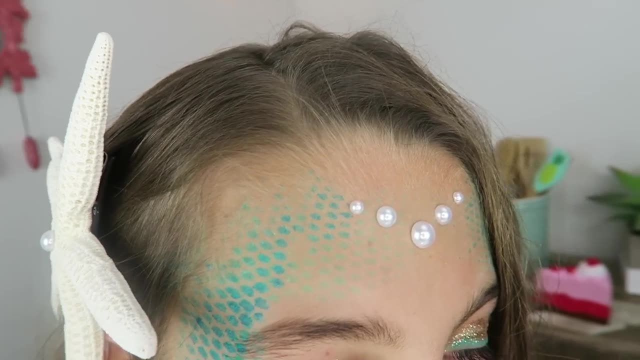 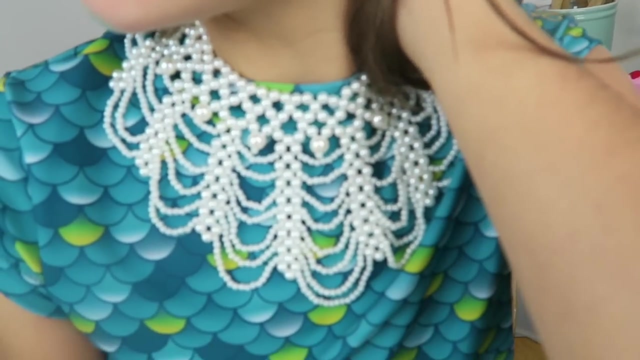 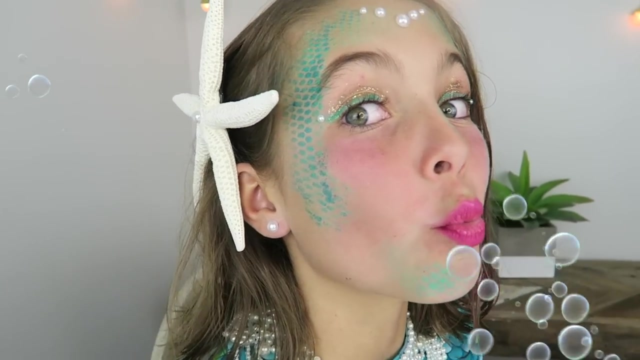 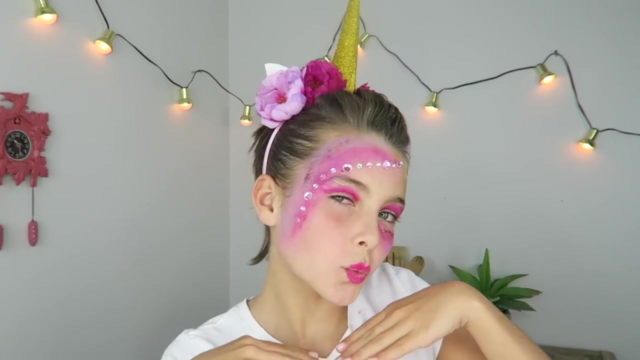 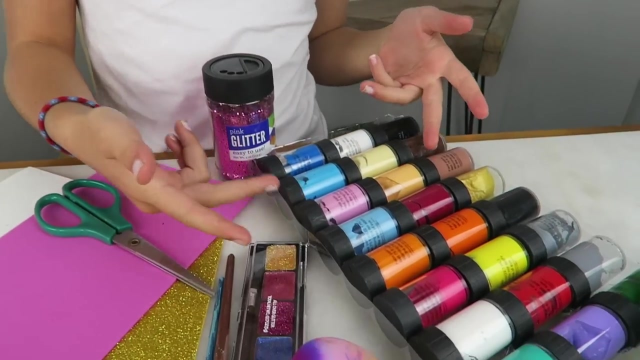 ready for some close-ups. I'm Ava, and today we'll be showing you how to make a DIY unicorn themed face for Halloween. look at all this cool supplies that we have. we have face paint, glitter, lots of glitter, scissors and even flowers. you can get these at my store and I'll see you in my next video. bye, bye. 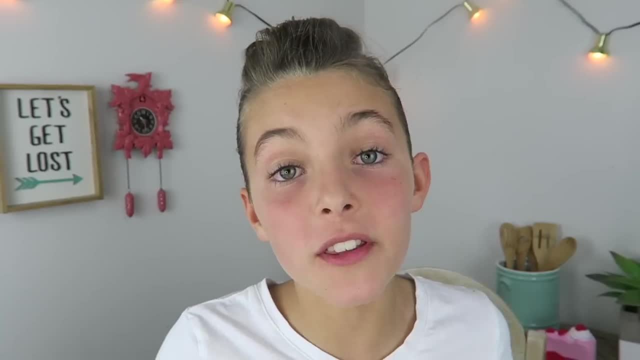 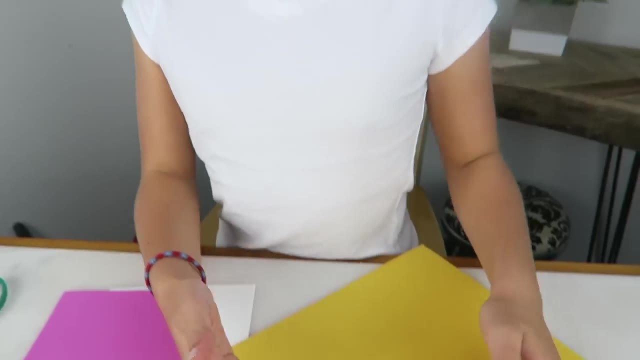 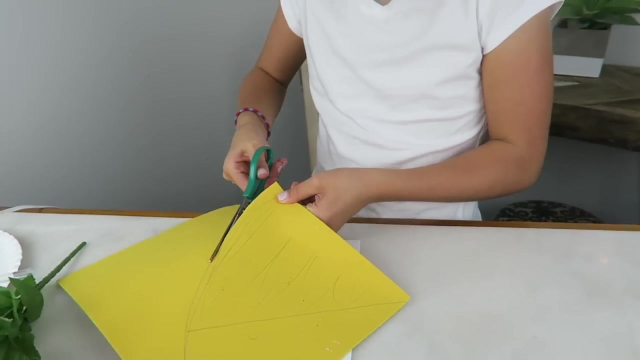 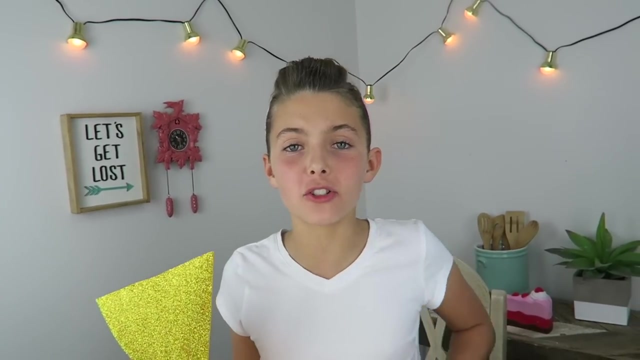 first I'll be showing you how to make the unicorn horn. so for this craft you need foam paper. I got gold glitter, white and pink, so I marked this gold glitter one with the shape of a piece of pizza. just gonna use my trusty little scissors. it kind of looks like a candy corn. oh, don't eat it bad, Tom Tom. so I'm gonna. 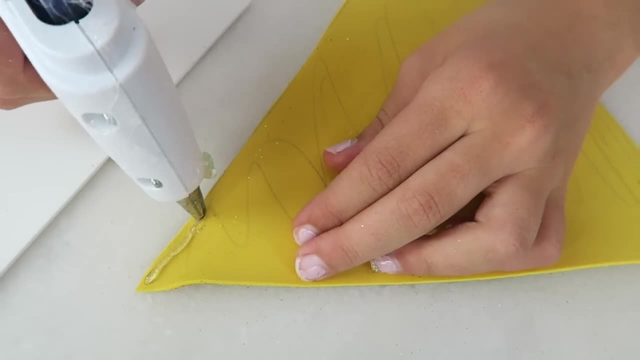 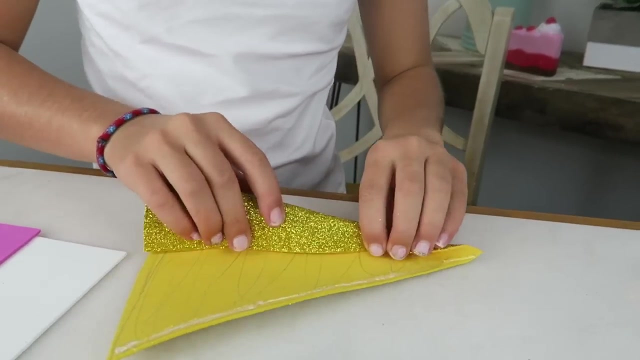 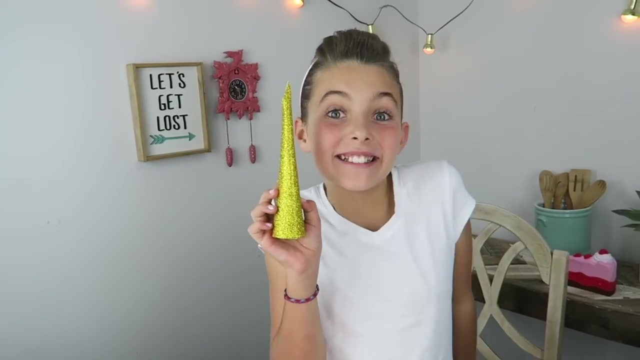 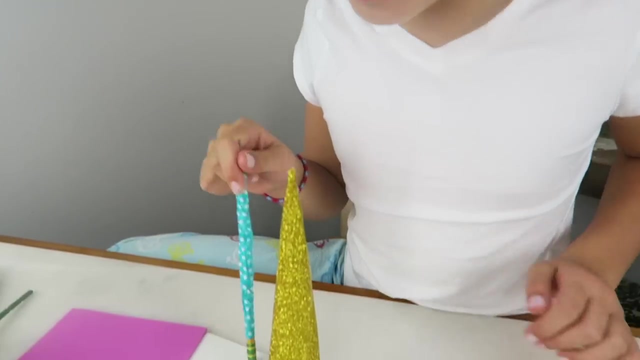 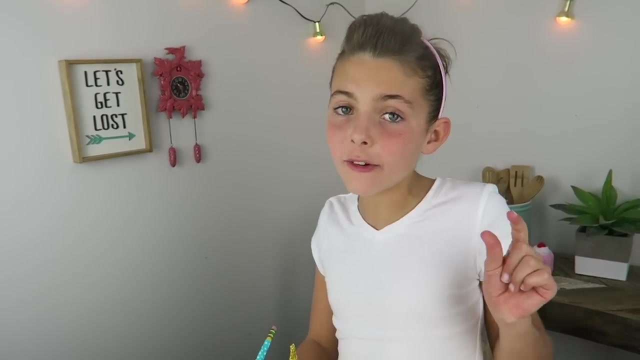 put a strip of glue all along one side of the unicorn horn. now I'm gonna roll it and hold it tight. ta-da, it's my little unicorn horn. so now you want to get your white foam paper and trace around the unicorn horn, but make sure that the circle is a little. 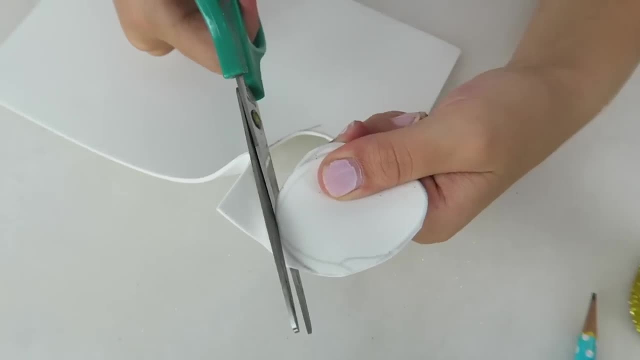 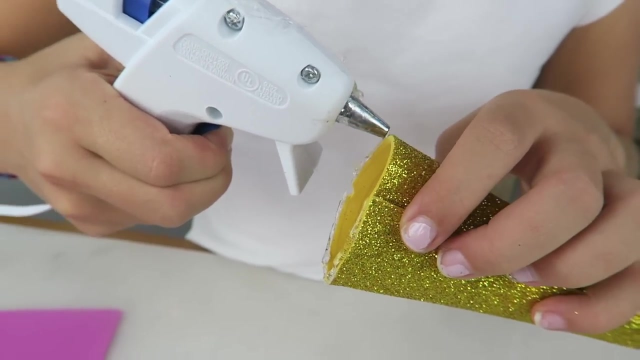 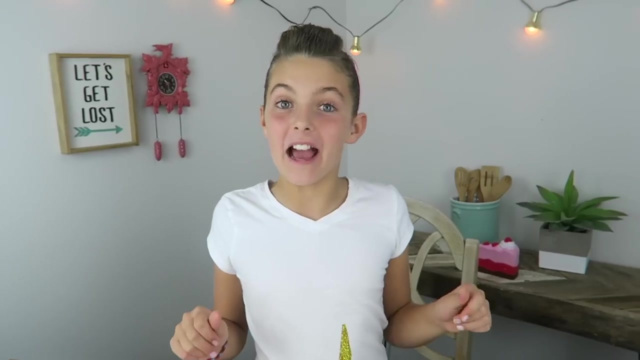 bit bigger than the base of the horn. so I'm going to put a little bit of glue on the base of the horn to make sure that the circle is a little bit bigger than the base of the horn. put some glue all the way around in there to get on. okay, now let's glue it. 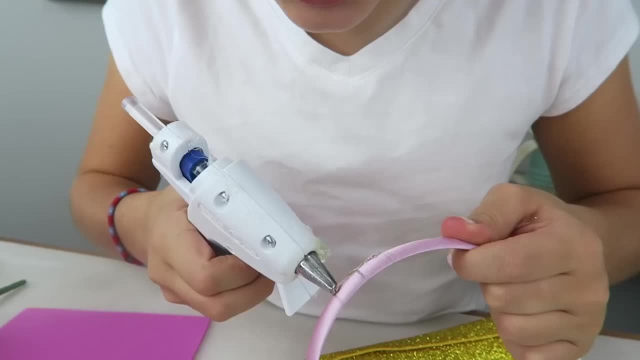 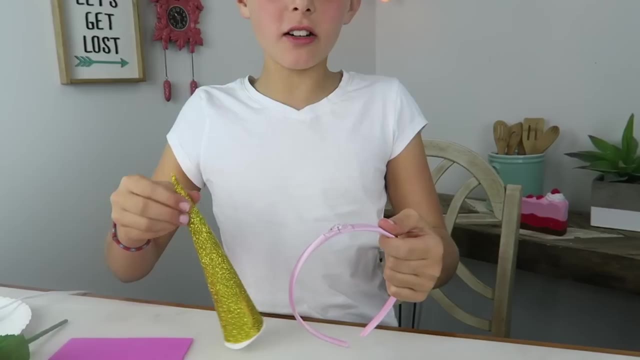 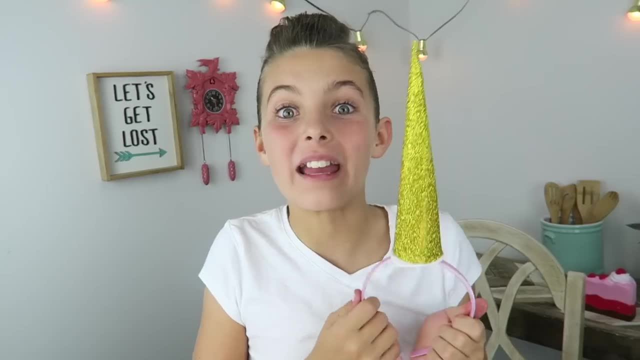 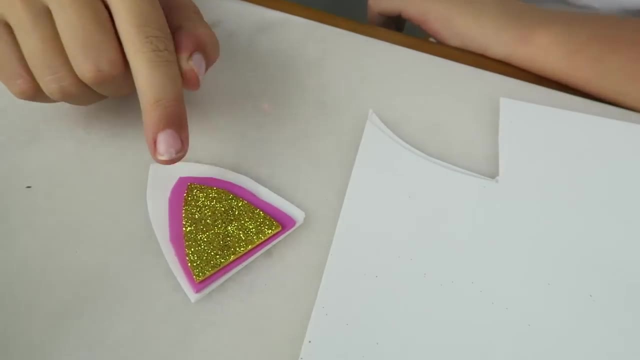 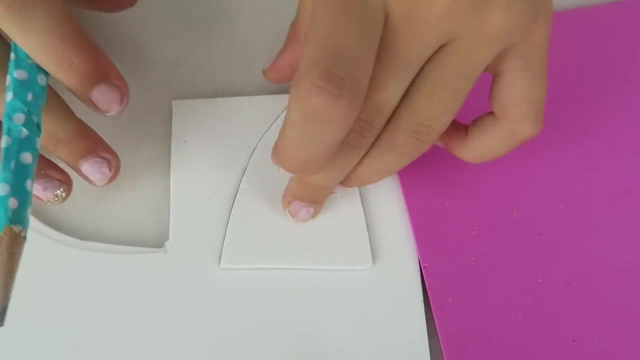 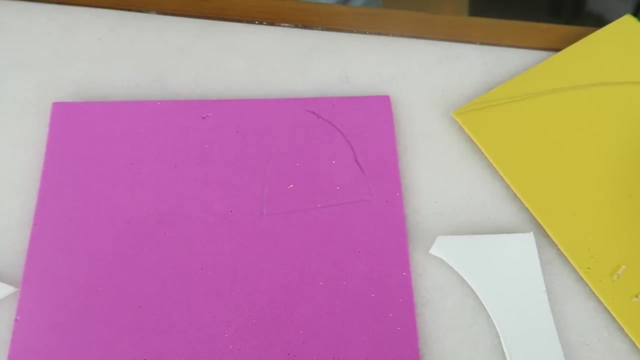 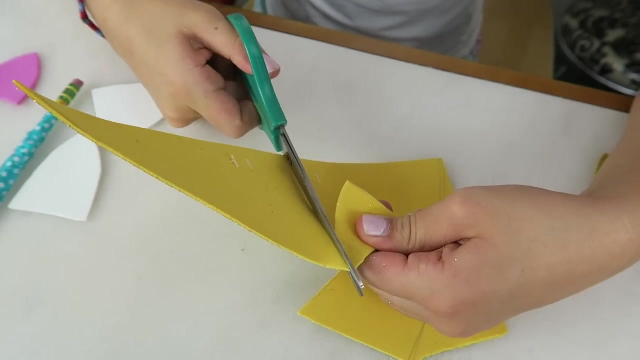 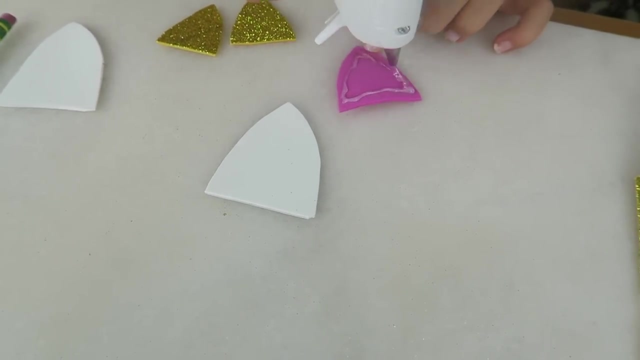 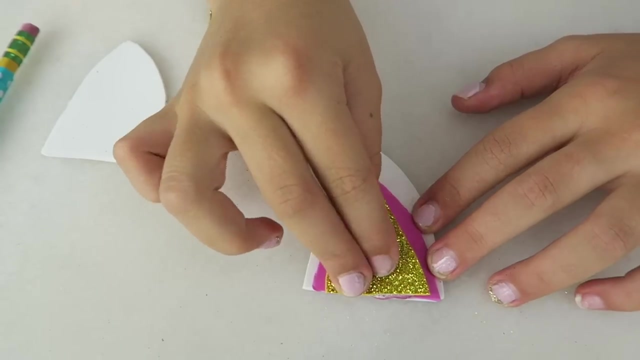 Okay, time for some ears. So we basically have three triangles: One white, one pink and one gold. Now I'm just going to trace it to make the second ear Next one. Alright, let's stack them up and glue them together. 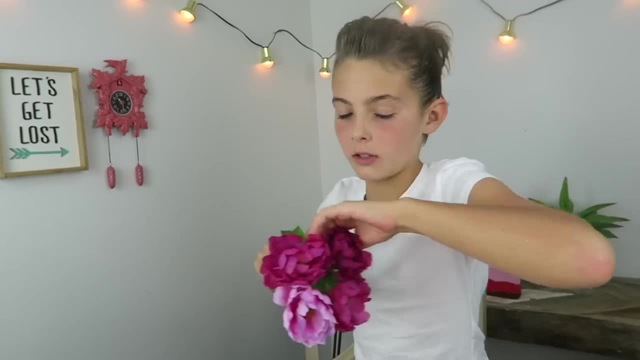 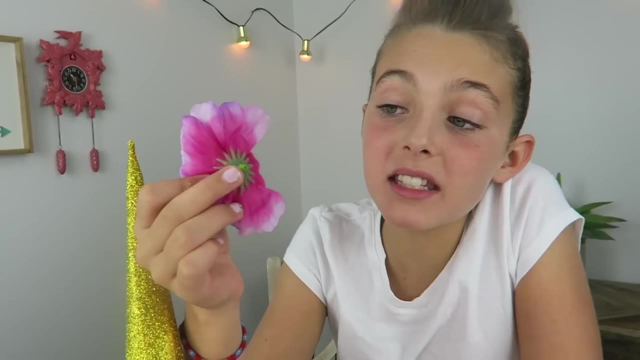 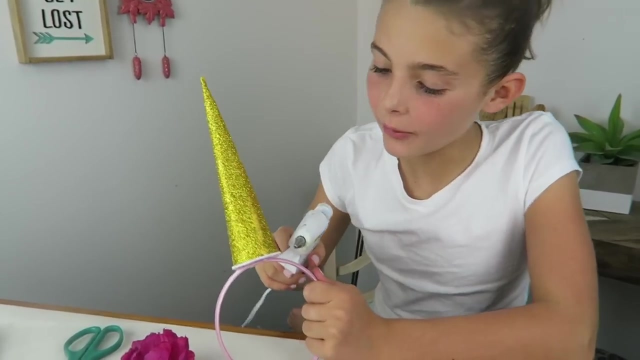 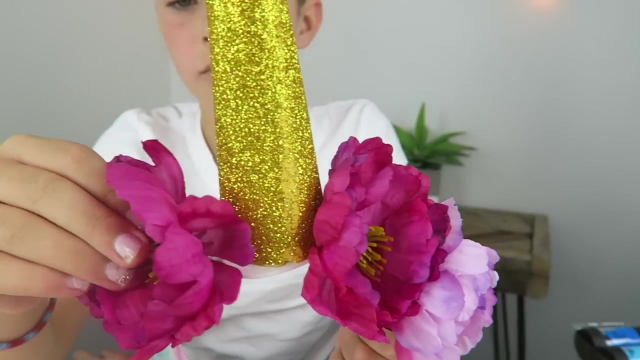 Alright, we've got to pop these babies off. Alright, Do you see this little nub on the back of the flower? We're going to glue that to the headband. We're going to do two flowers on each side. Now do the other side. 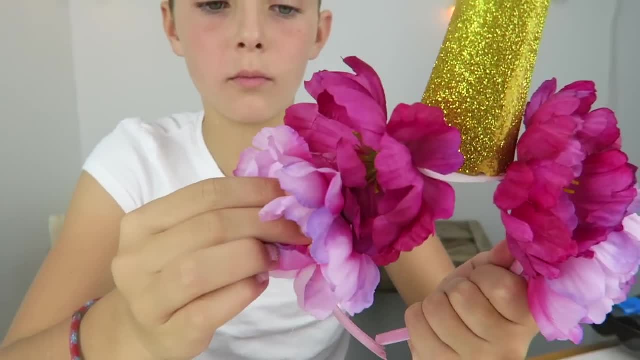 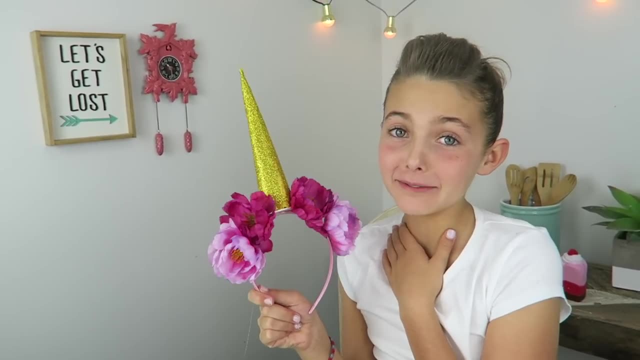 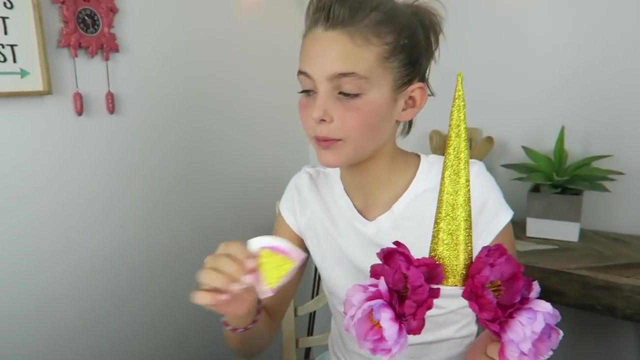 It looks like a flower. It looks so pretty, Let's put these ears on. I'm going to glue the ears right in between the two flowers, Just like that Trusty glue gun. We need more glue. We need more glue. 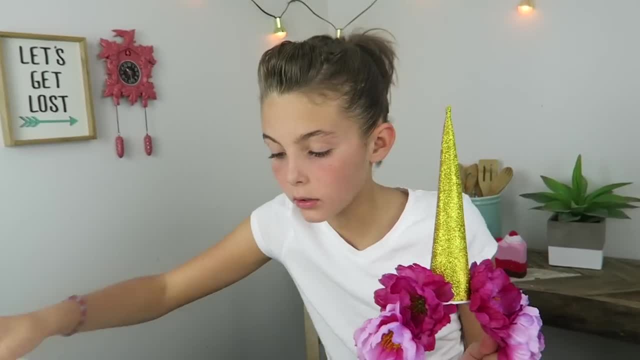 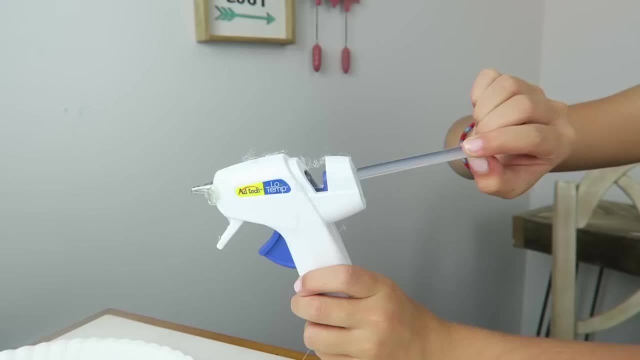 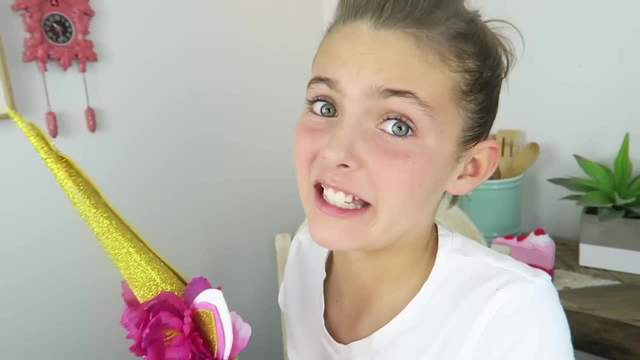 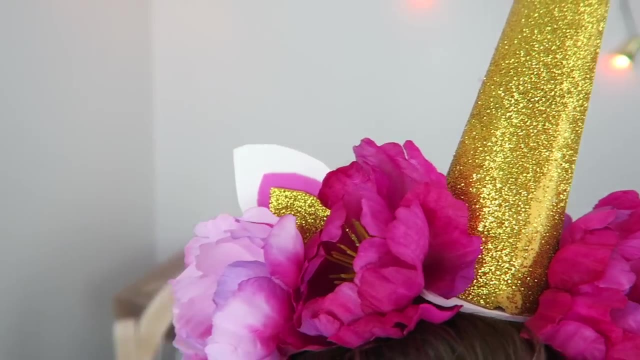 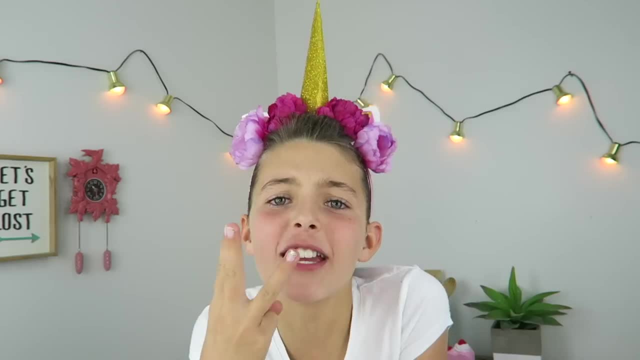 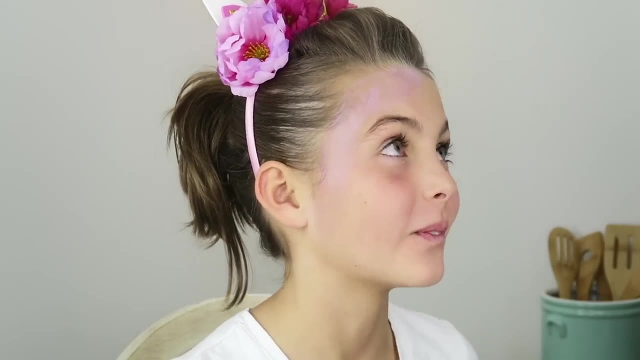 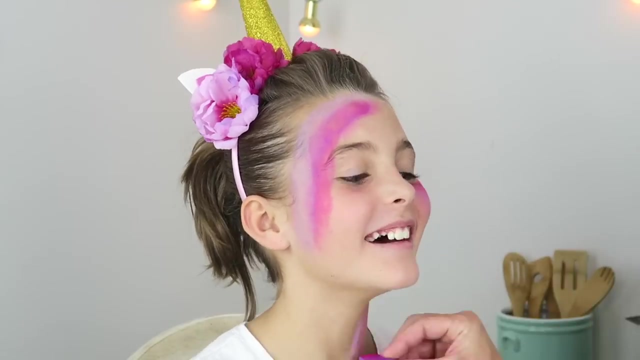 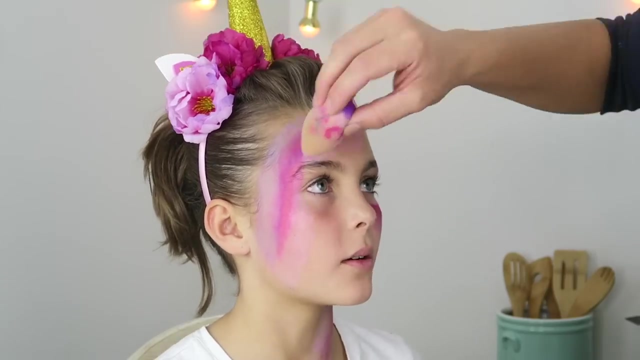 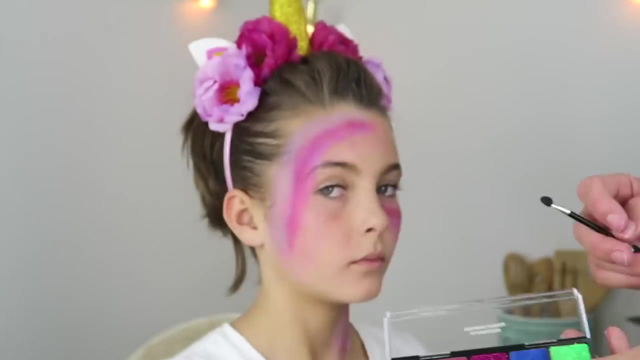 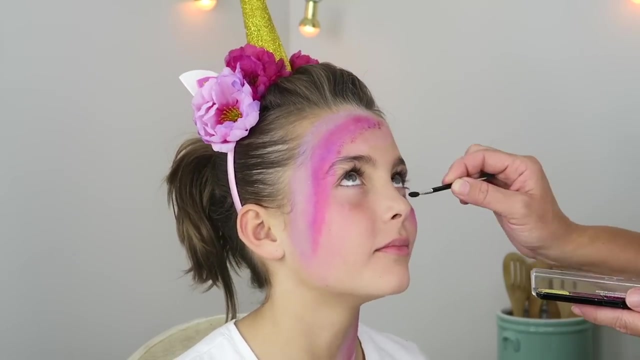 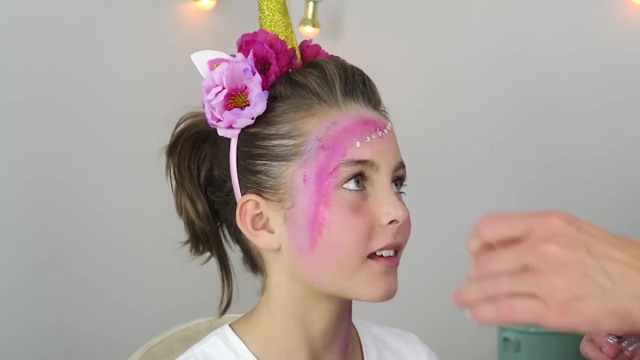 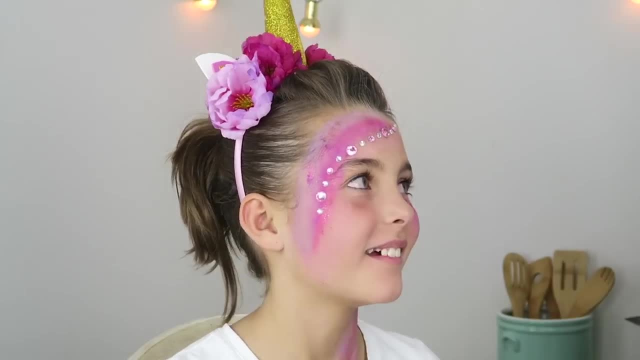 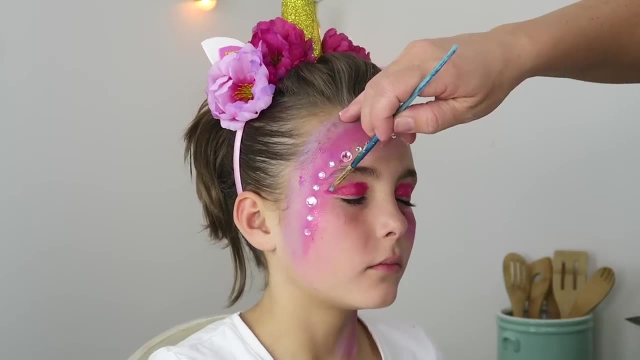 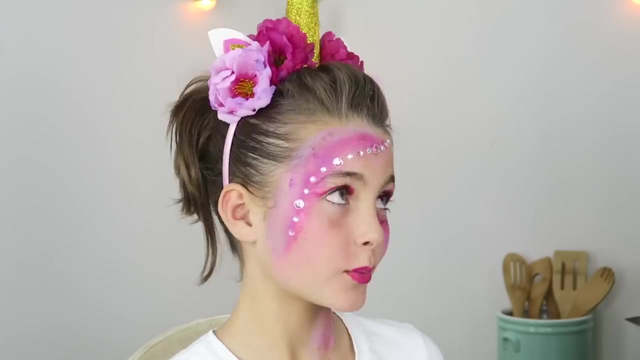 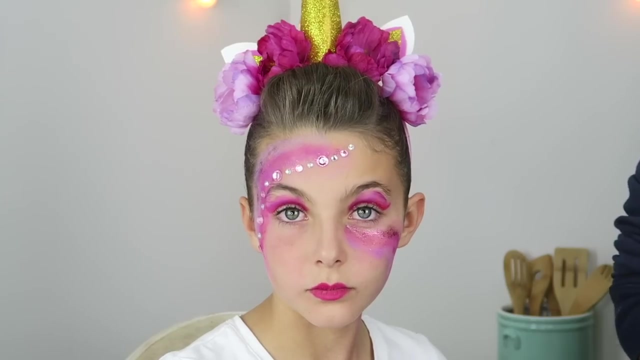 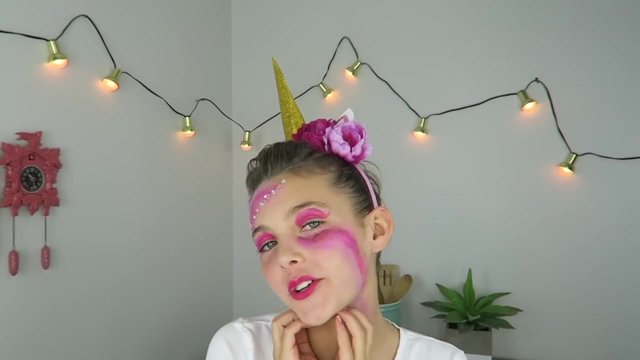 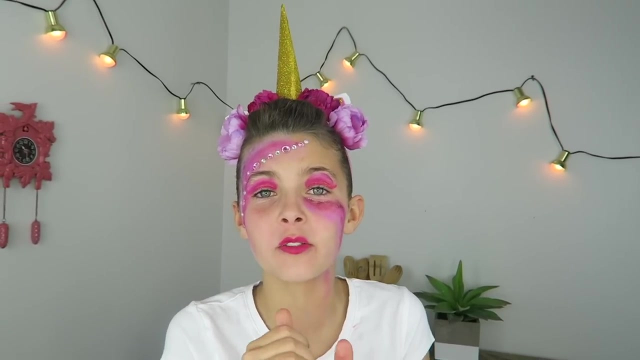 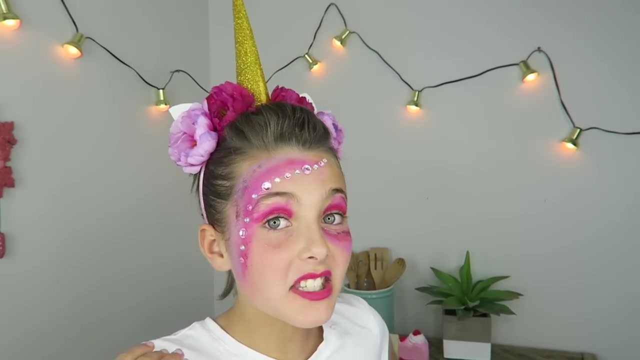 After a while I'm sensing a smile. Voila Do I look like a true unicorn. This DIY does not include how to make hooves. You can just make fists. Now it's time for the ultimate close-up, so you can see all the deets. 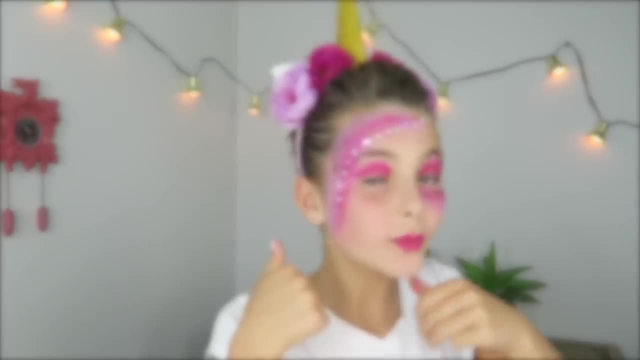 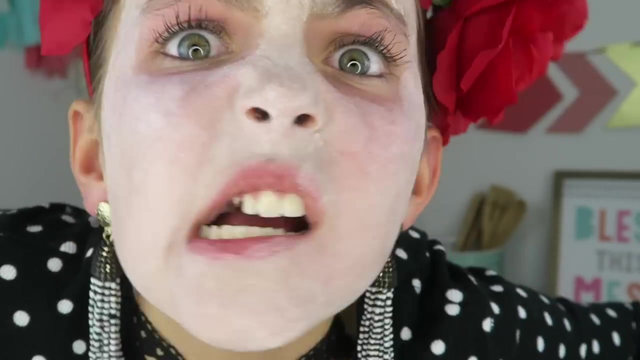 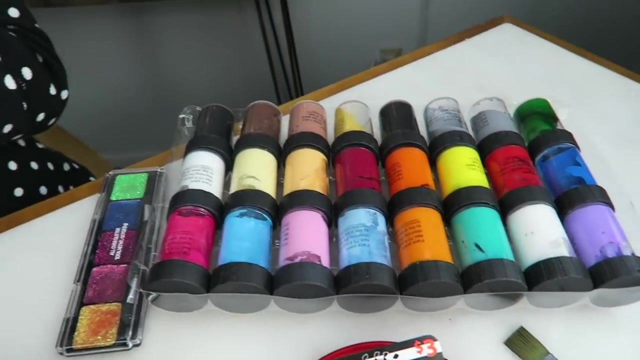 I'm Ava, and today I'll be showing you how to make a DIY Day of the Dead Halloween costume with a makeup tutorial. Look at all these amazing supplies that we have. They are so gorgeous. We will be making the headpiece first. 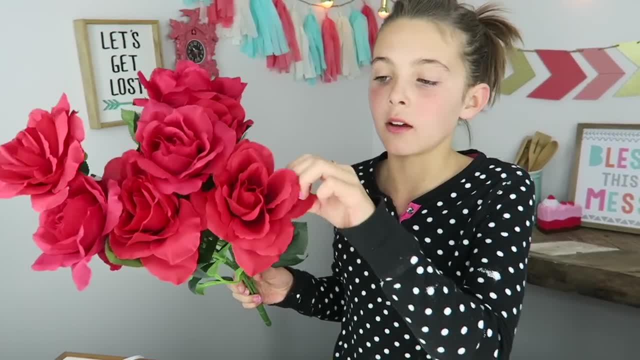 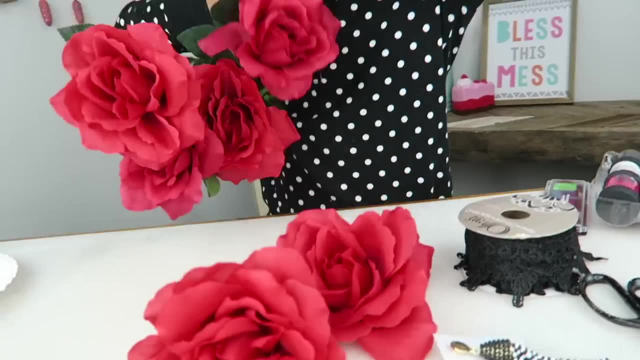 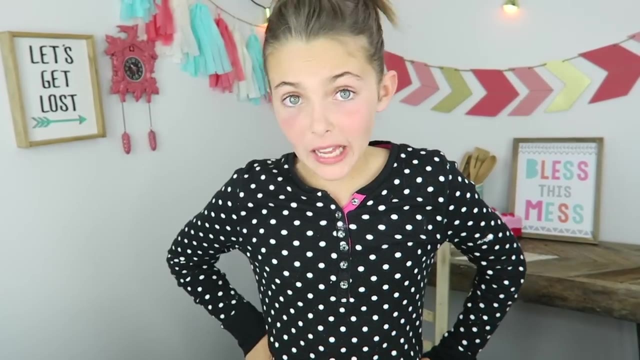 So what you need is some red fake roses, and I'm going to use five, so just like, pop them off the stem. We don't need these, Okay? so then you need a red headband and you also need a hot glue gun. 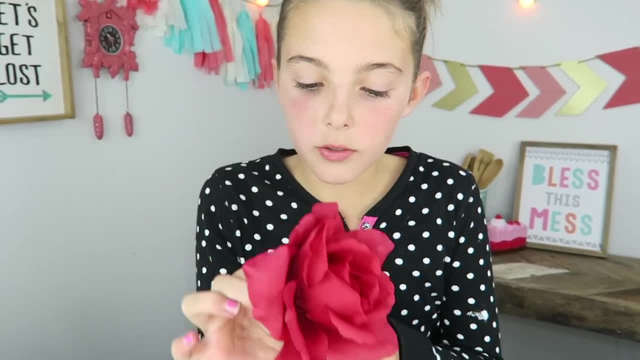 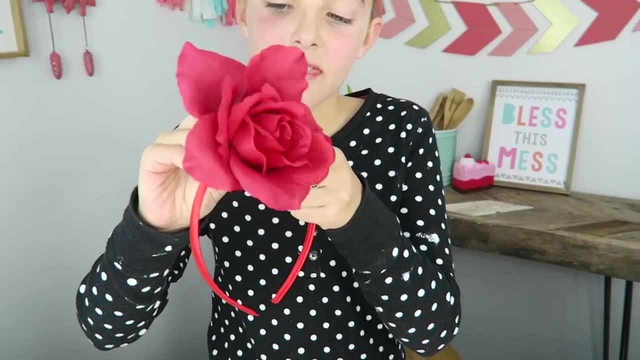 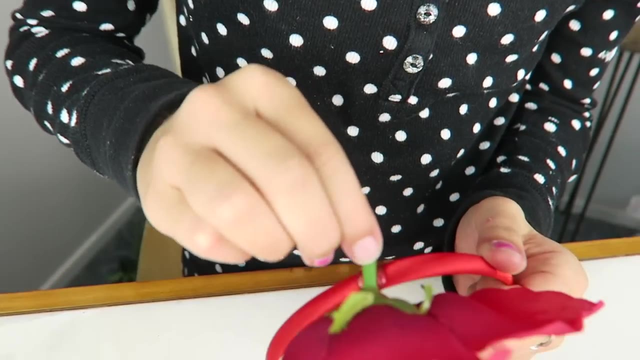 This is what we're going to do. You're going to grab a red rose and you're going to hot glue it. so it's like, right in the center of the headband, Point it forward just like that, Hold it down until it dries. 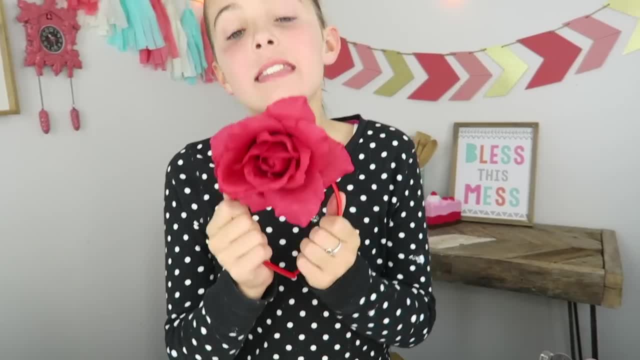 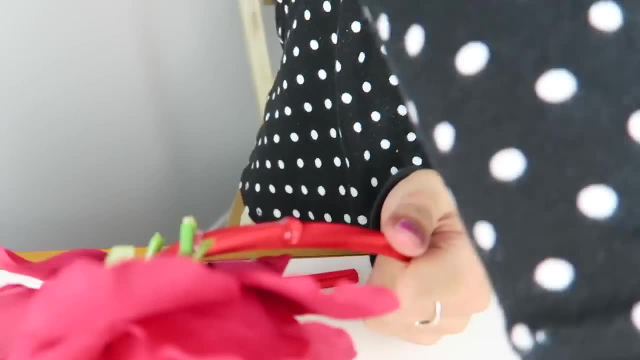 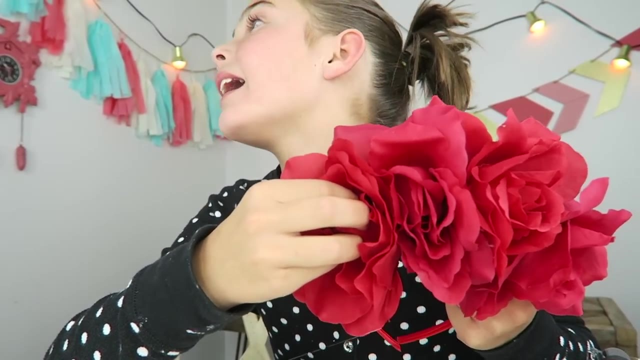 Okay, now we're going to put some of the other flowers all around it. I just have to be patient and let it dry. let it dry, Can't hold it back anymore. Okay, I'm sorry, I'll stop. Let's see how it looks. 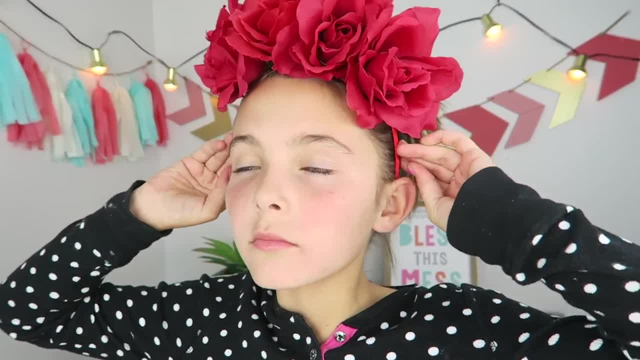 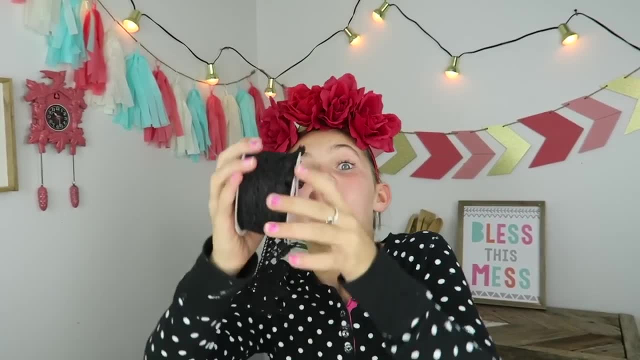 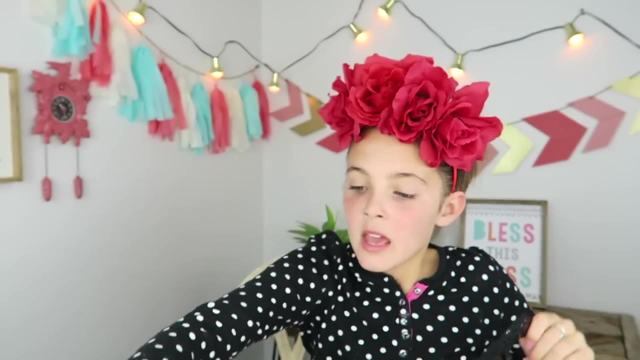 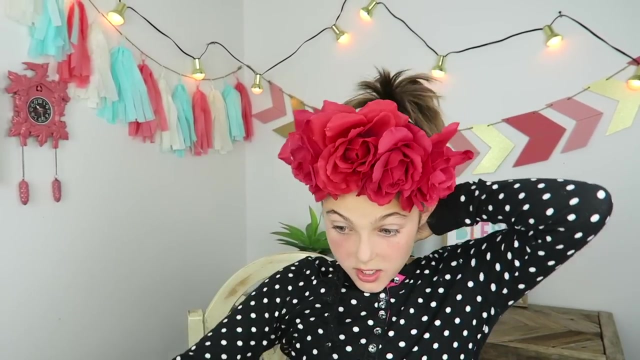 On to the necklace. So I found this black lace stuff. It has a beautiful pattern and I'm just going to measure the length. well, around, I'm just going to go. oh, this is harder than it looks, I'm going to cut it. 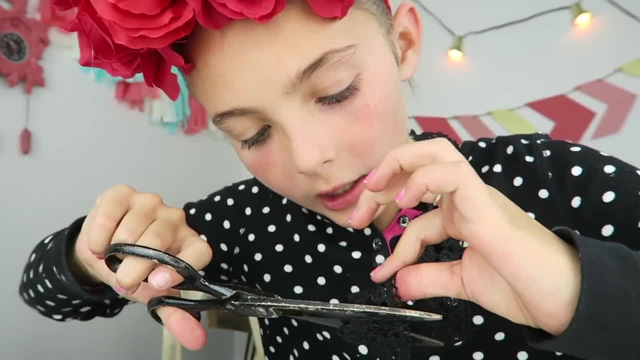 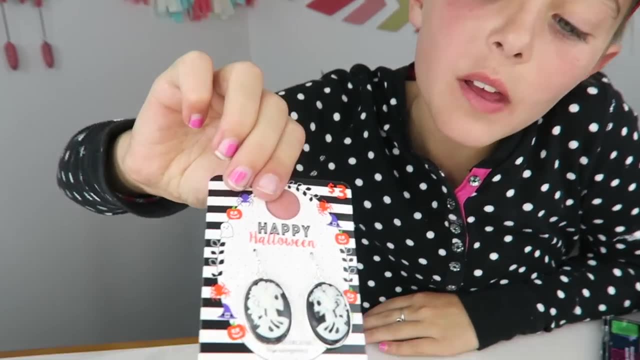 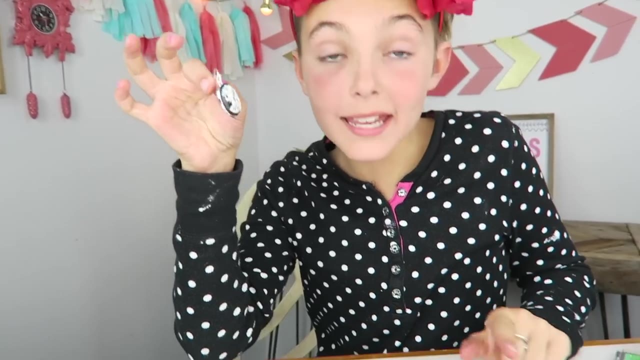 Just, I'm just going to cut it a little longer than the length of my neck there. and then I got these adorable earrings. they have skeletons on them and I'm just gonna take one of them and I'm gonna hook it right in the middle of my choker and then pinch it. 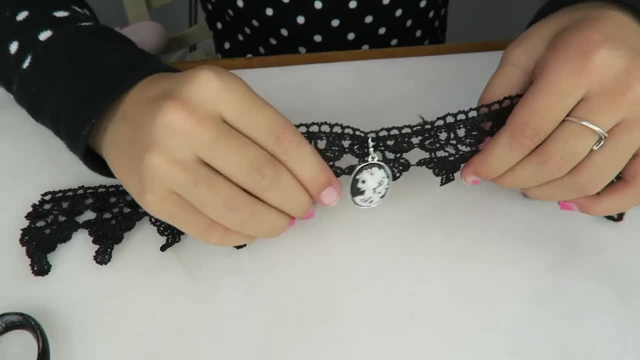 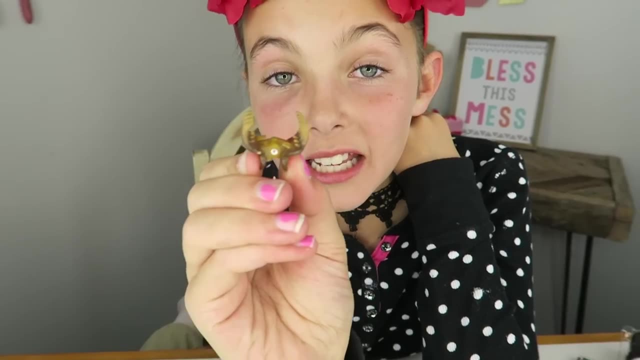 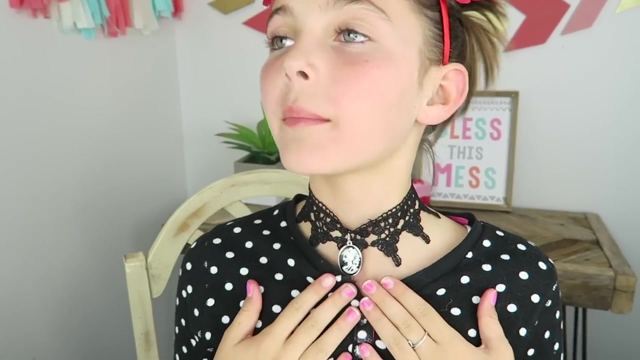 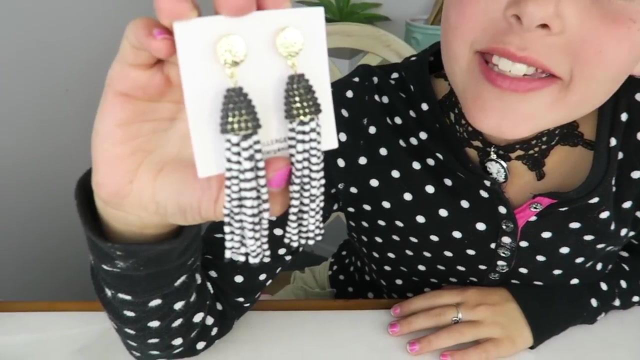 shut on the back. voila, our very own choker. now you're gonna wrap it around your neck and then you're gonna get a hair clippy and clip it so it doesn't move- voila, do you like my choker? so I found these really cool earrings at 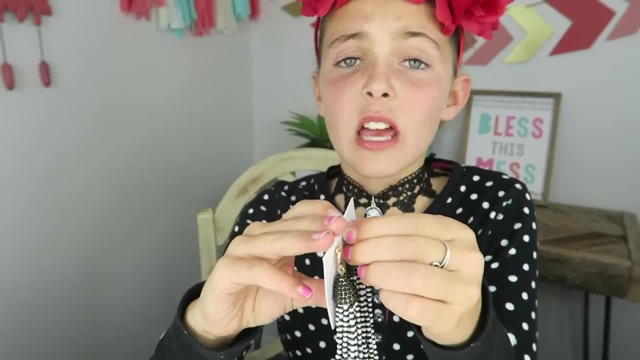 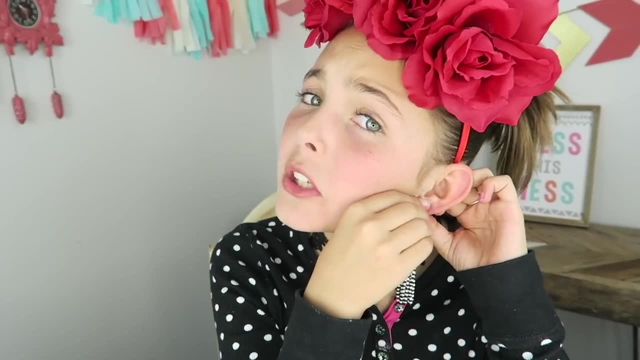 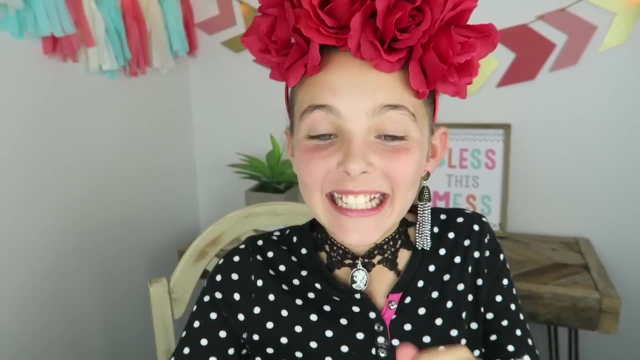 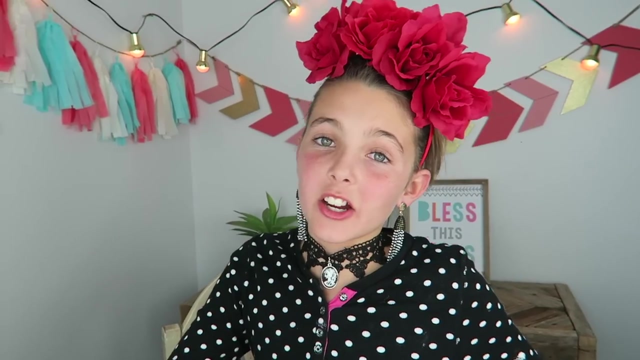 Walmart. they are so cool, so I'm just gonna use them as normal earrings and put them in. do you have your ears pierced? comment down below. if you don't, you can just use clips. well, these things are heavy. I've never worn earrings this big. okay, there we go. so I looked in the mirror and decided that I want to add. 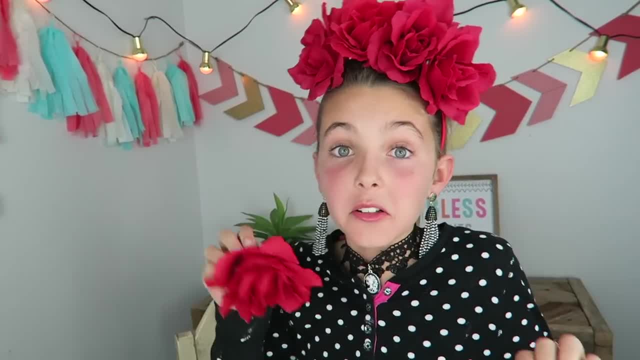 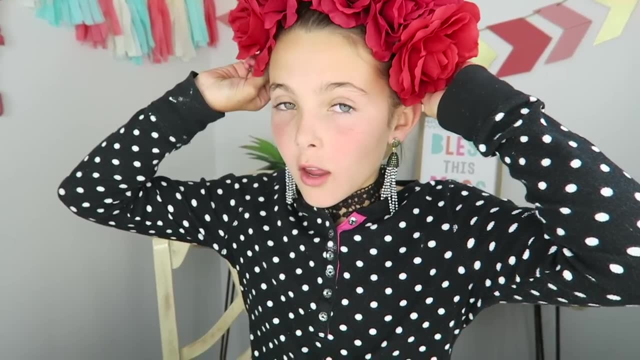 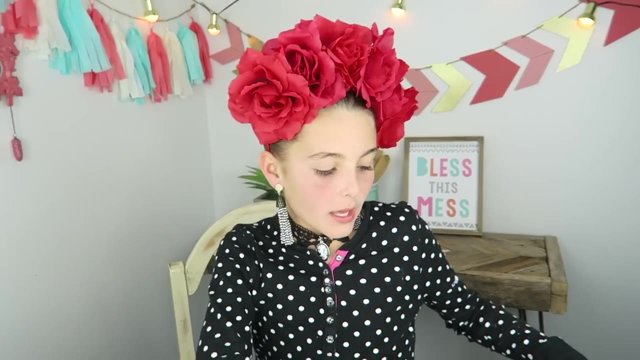 two more flowers to my headband, so let's do it. voila, is that better? okay, now it's time for the makeup. so I'm gonna put on my headband and then I'm gonna put my makeup on. so we have a whole bunch of face paint, glitter, mascara, paintbrushes. 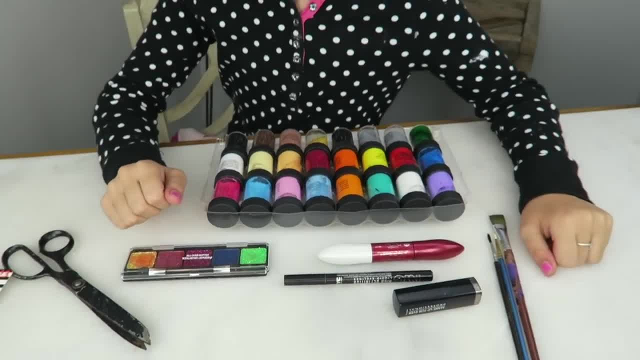 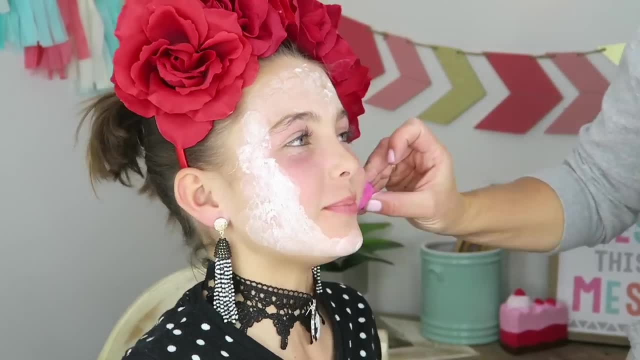 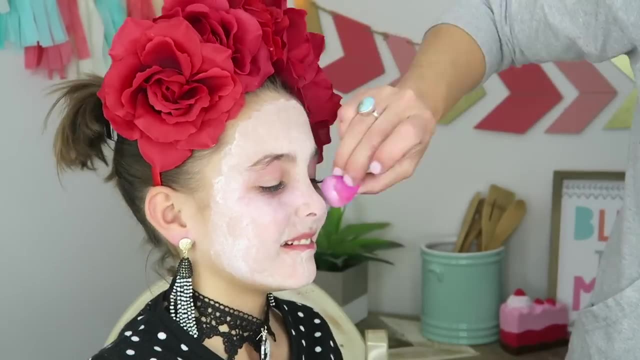 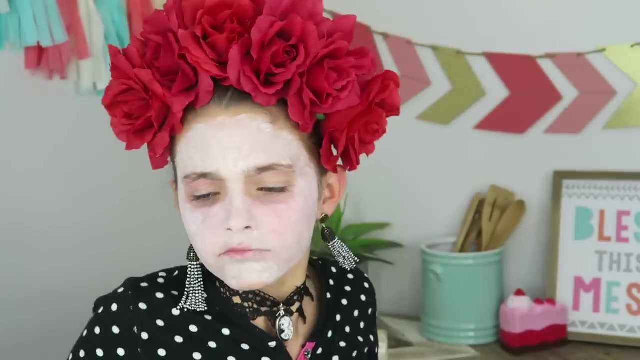 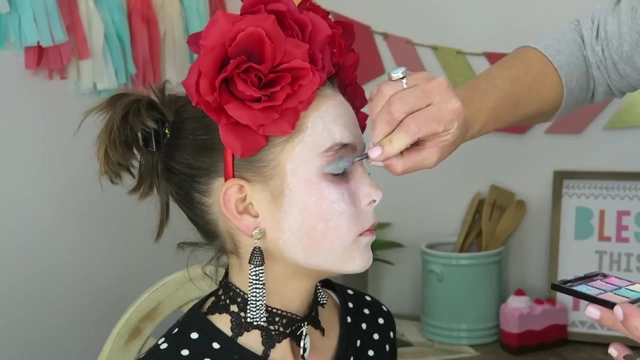 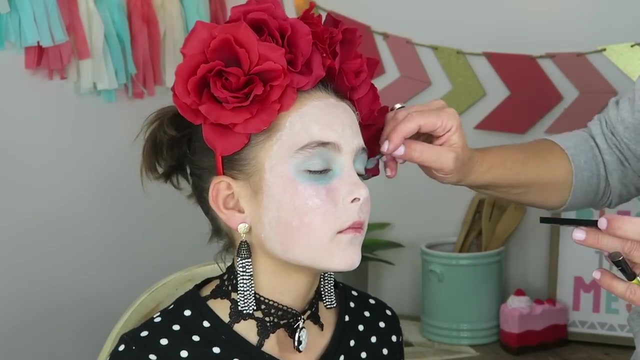 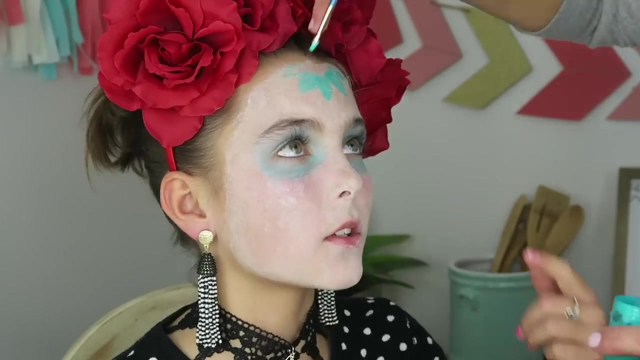 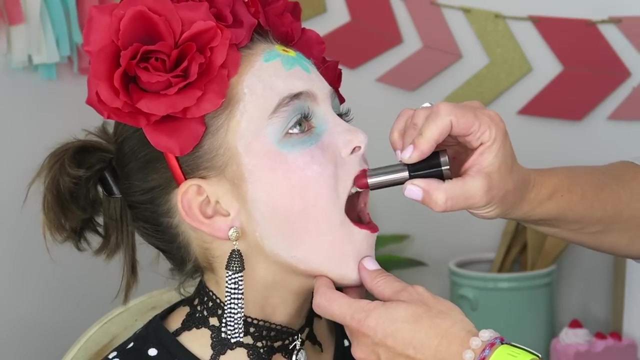 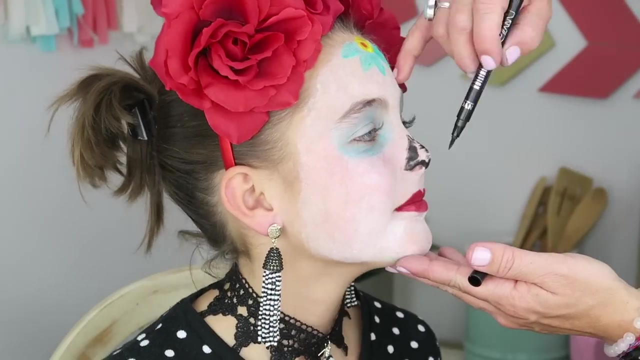 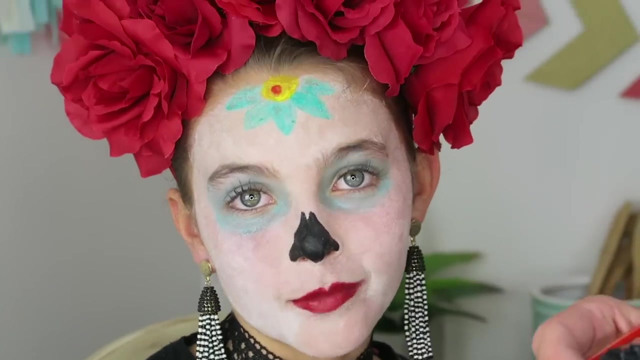 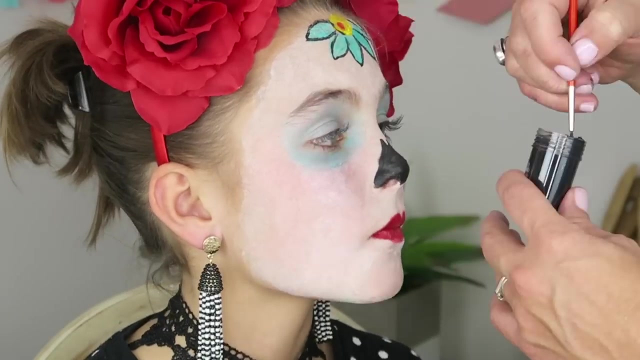 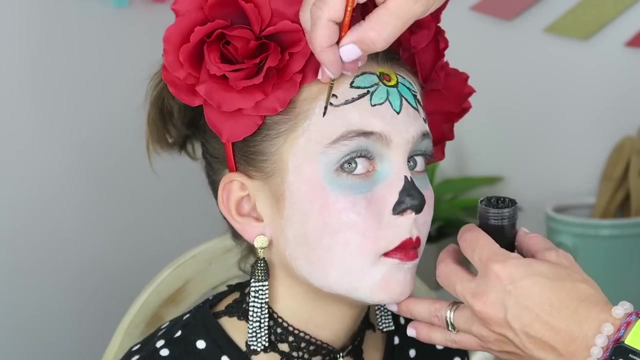 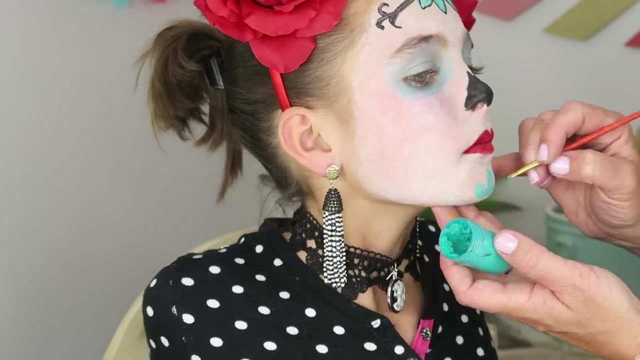 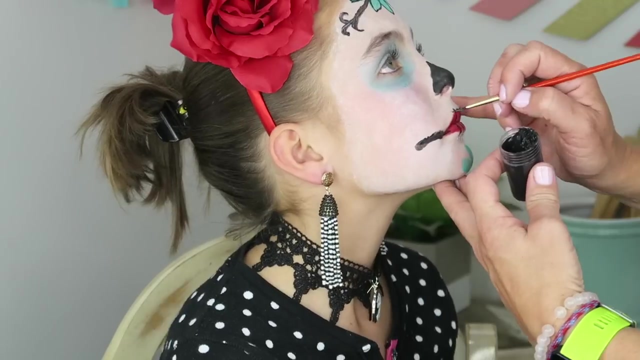 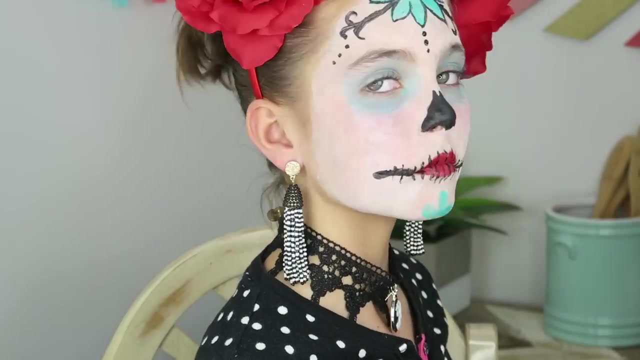 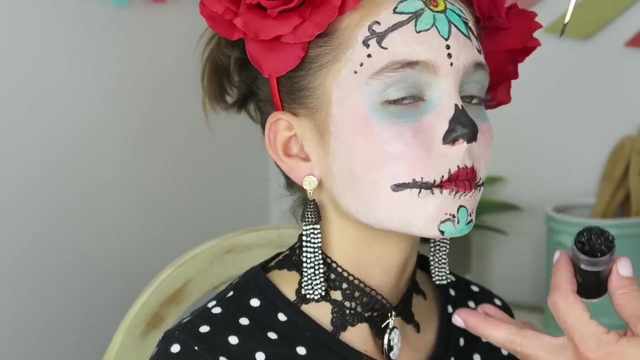 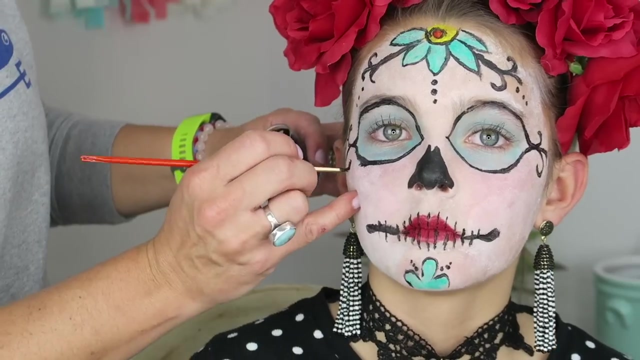 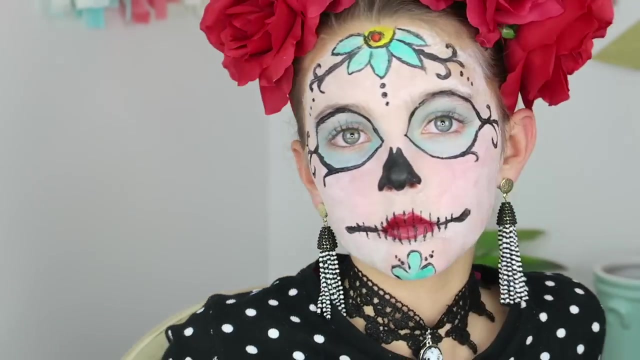 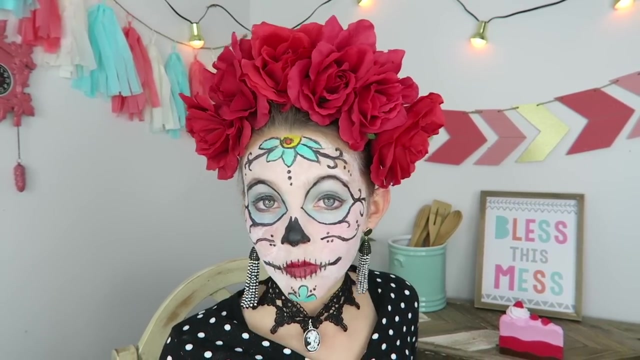 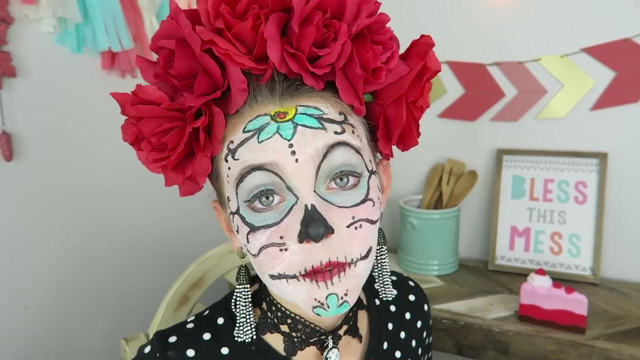 eyeliner and lipstick. so let's do this thing: three, two, one, three, two, one. Thank you, Thank you, Thank you. How does it look? Does it look spook-tacular? You don't have to do the face paint, just like ours. 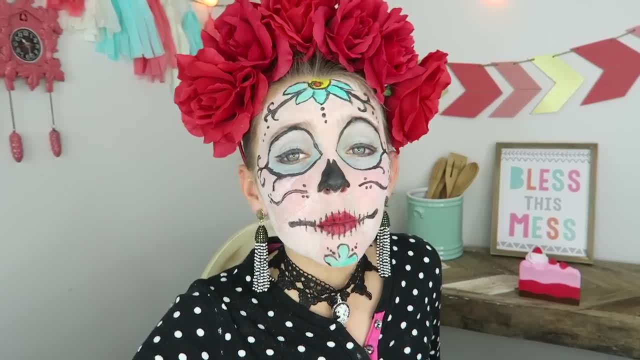 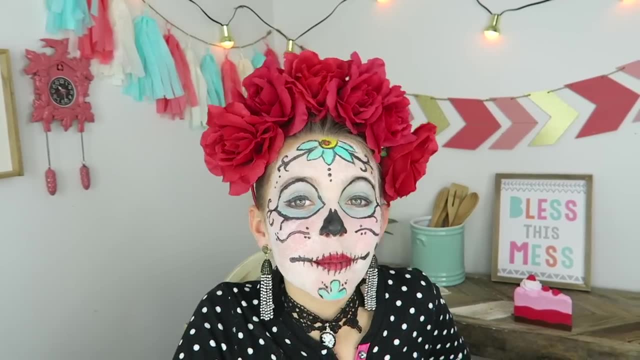 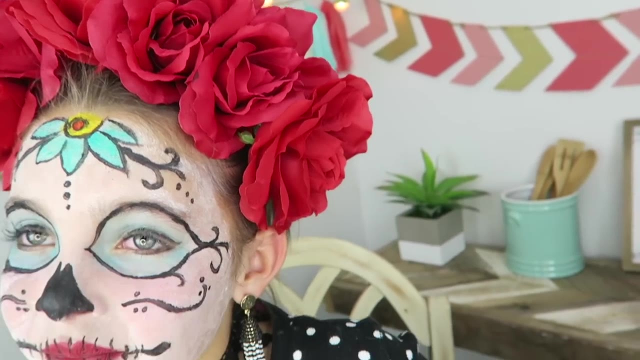 Be creative, Like: do whatever you want. On mine, we did a. we did a lot of flowers and swirlies and dots, A lot of them. Alright, guys, here's some close-ups. Ready set go. I'll be showing you how to make. 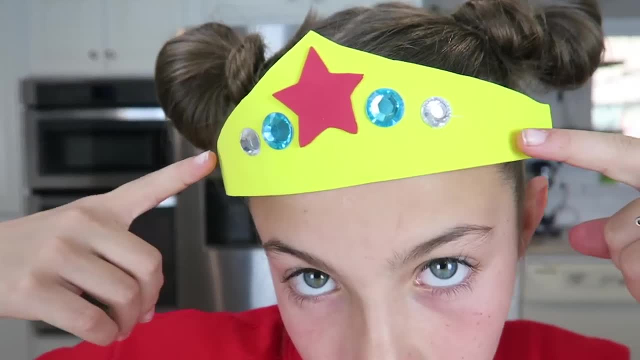 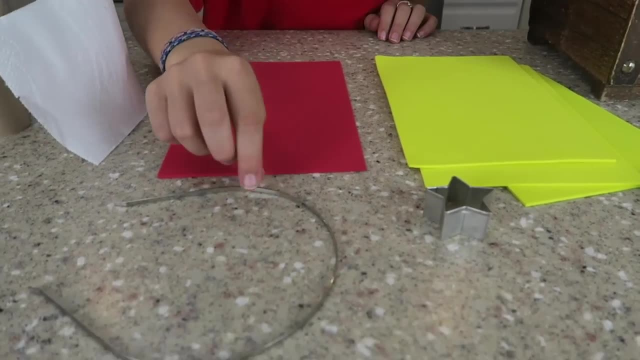 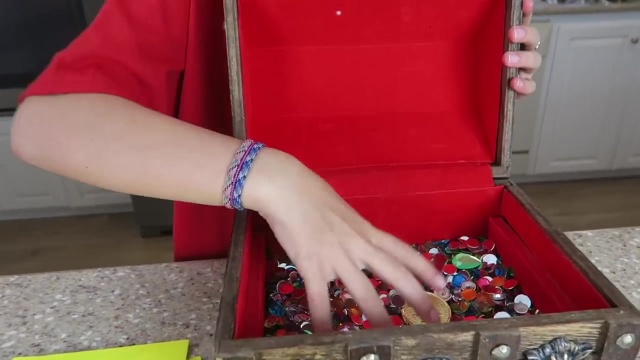 a DIY Wonder Woman cuff bracelet and headband. The things you will need will be two toilet paper rolls, red and yellow foam paper, a headband, a star stencil, some scissors, a hot glue gun and some jewels. You want to grab your pencil. 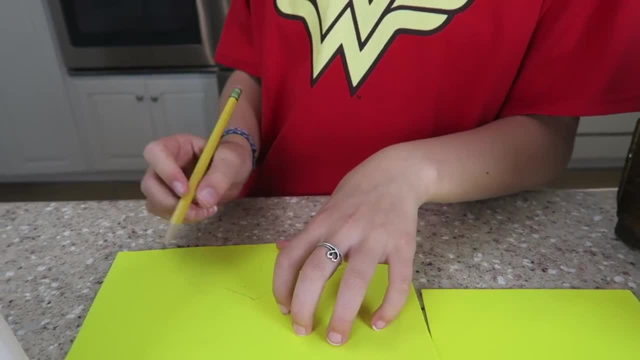 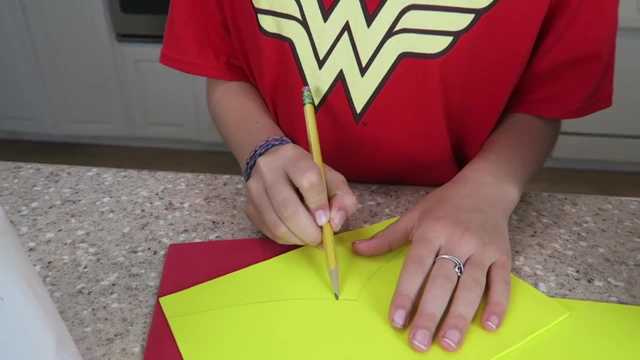 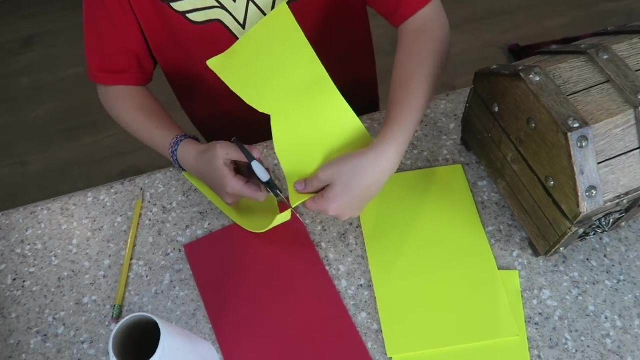 and your yellow foam paper You kind of want to make like a mountain shape. See how her headband kind of comes up and then back down. That's what I'm doing right here. Okay, carefully, just going to cut it out, Alright. 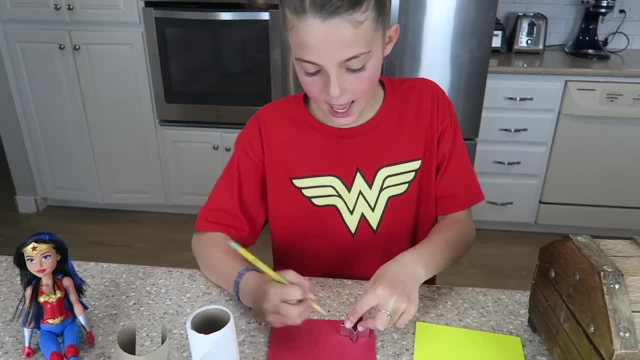 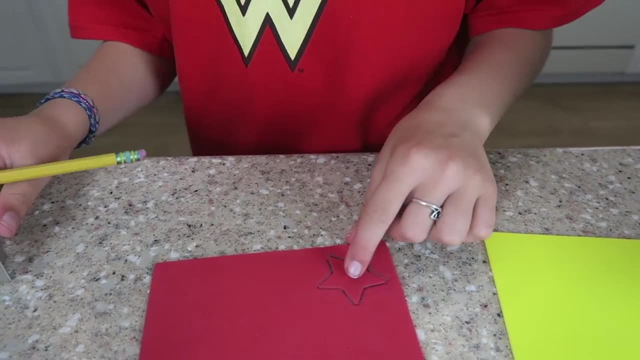 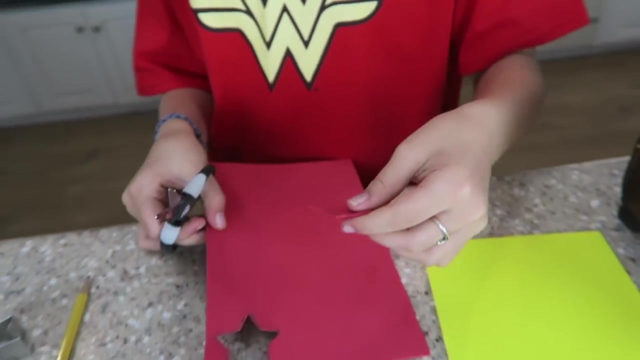 See, It's like a little headband. Now I'm tracing the star stencil. Whoa, that looks cool. Alright, now let's cut it out. There we go. we have a little star. Now I'm gonna grab my low temp glue gun. 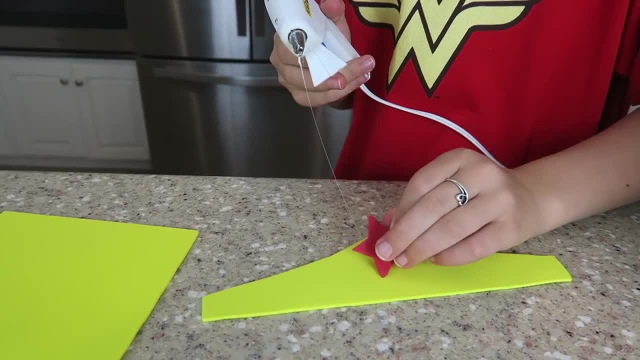 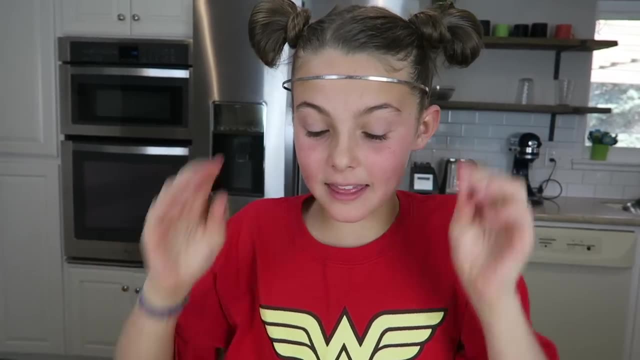 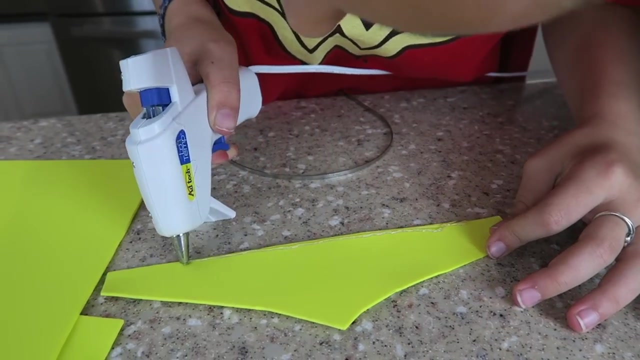 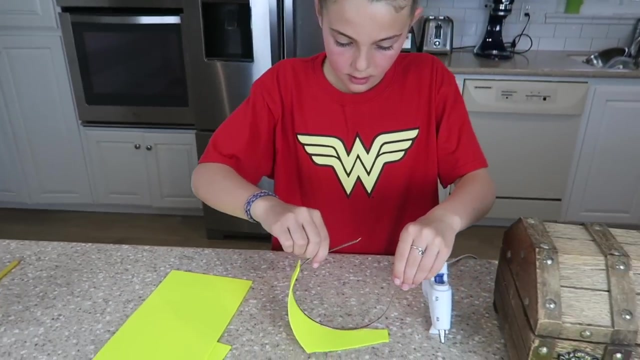 and glue the star down. Alright, this is how you're gonna wear your headband. Gonna wear it like this. and then we're gonna glue this right there, Ta-da, And I'm just gonna roll it like this back and forth. 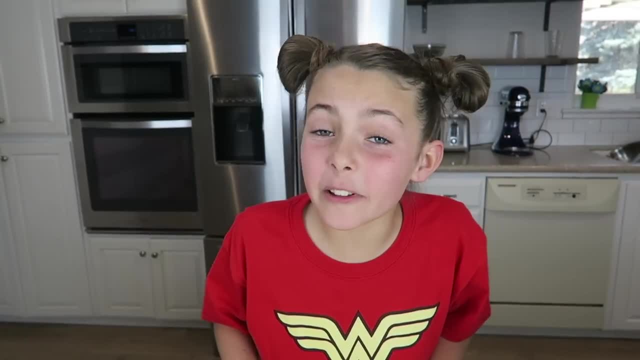 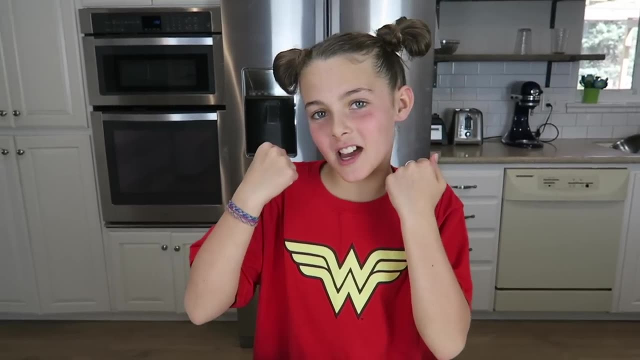 There we go. That was easy, huh, You don't want to put the headband on right away or else it will stick to your head. And now we're gonna make her bulletproof cuffs. But they're not actually bulletproof. 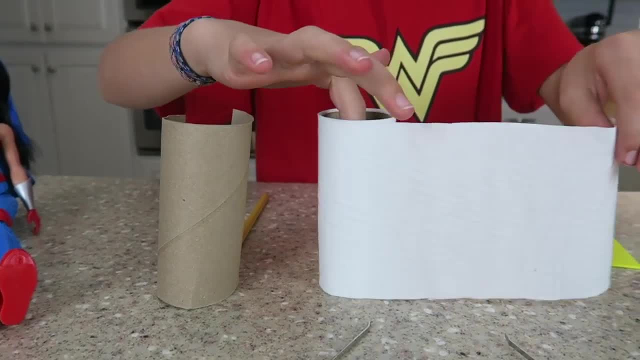 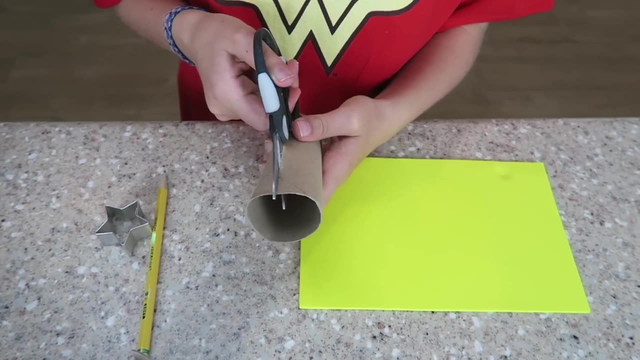 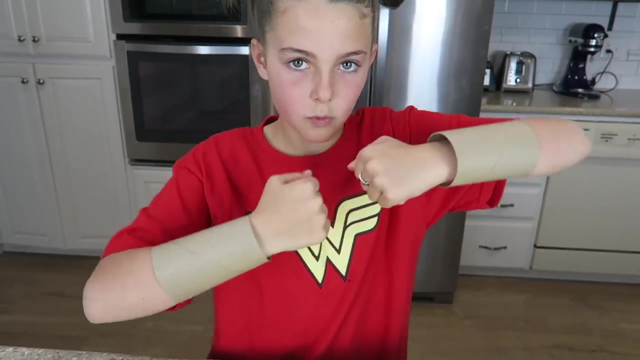 it's just paper, foam paper. Get your empty roll of toilet paper and cut it right down the middle. Alright, there we go. See, check it out, It goes right on my wrist. Now we're gonna cover them in yellow foam paper. 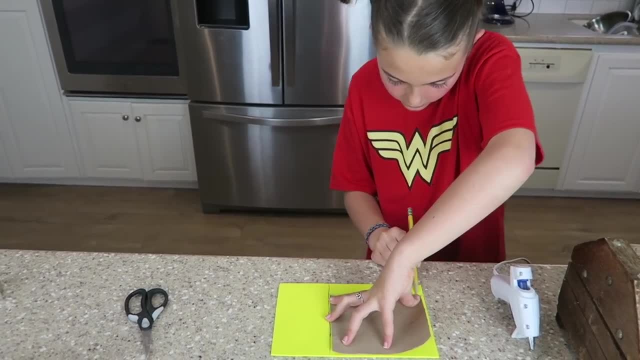 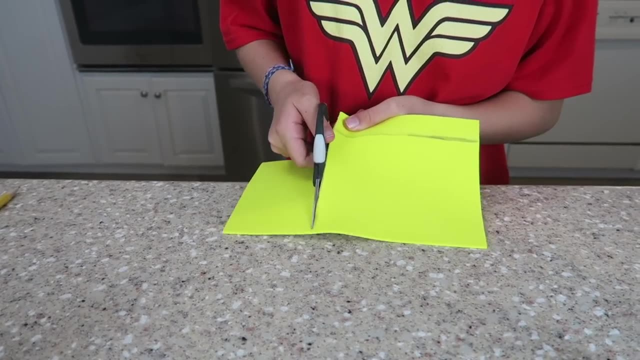 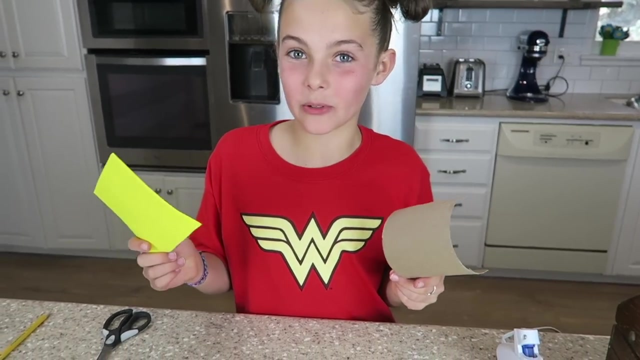 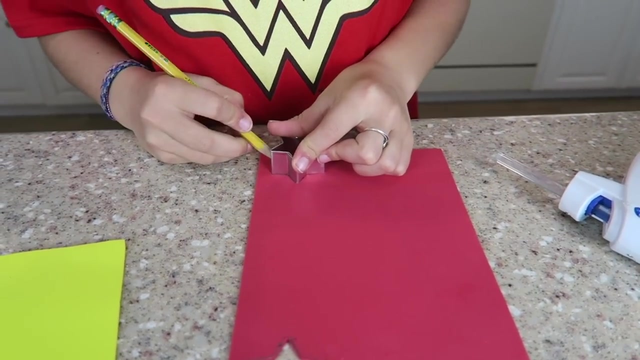 Alright, I'm just outlining them. Alright, and it's. we're outlining this roll of toilet paper, Then I'm gonna cut it out. Now, it's the same size I like toilet paper roll. Let's cut out two more stars for our cuffs. 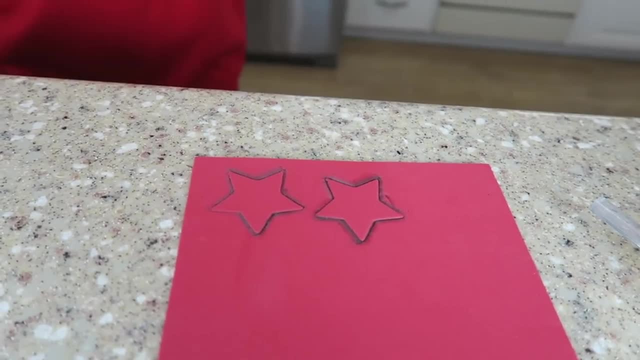 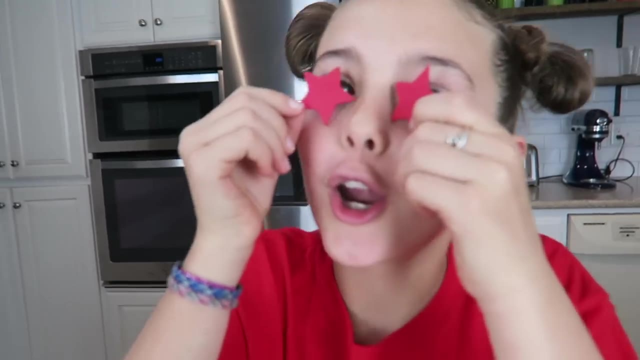 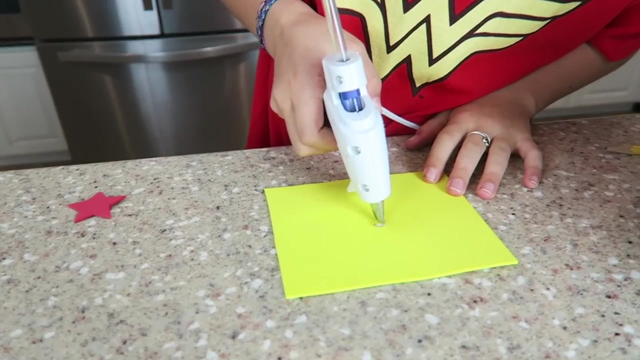 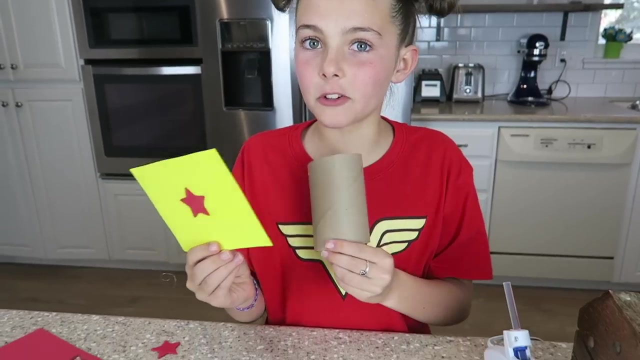 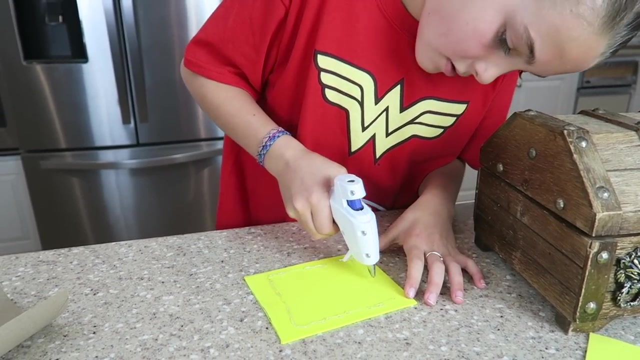 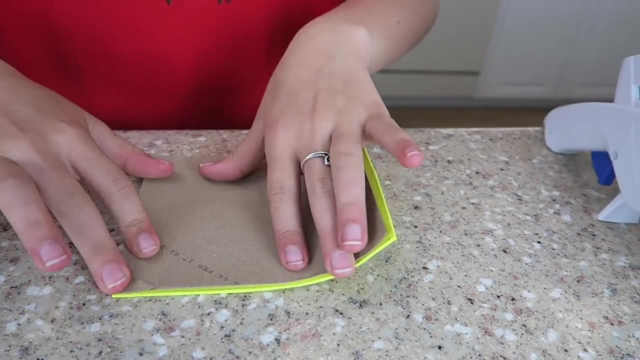 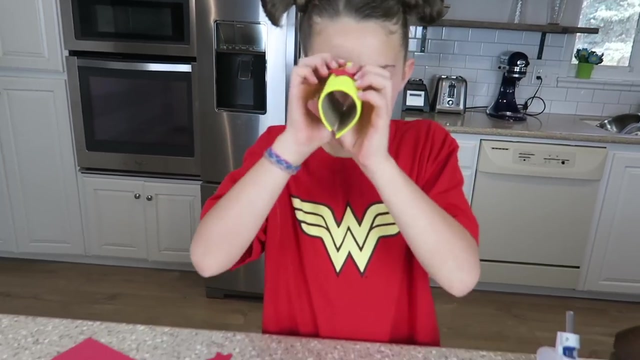 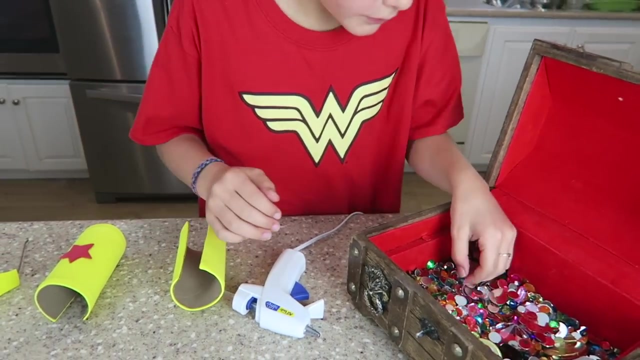 Okay, there we go, let's glue it on. I'm gonna put it right in the middle. now let's glue it on our paper roll. okay, just gonna go like this, and then you just want to make it into its world form again. now we're just gonna add some bling, hmm. 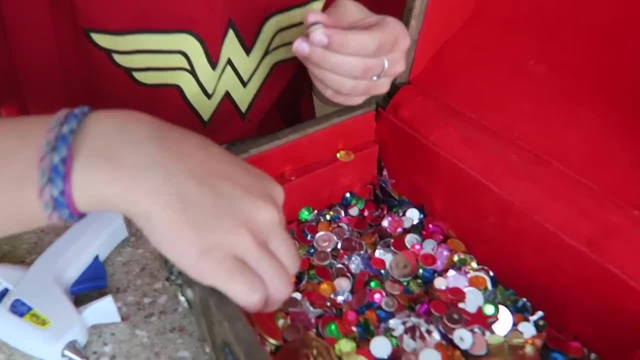 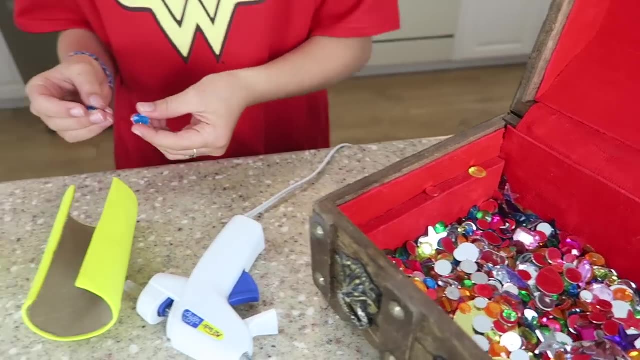 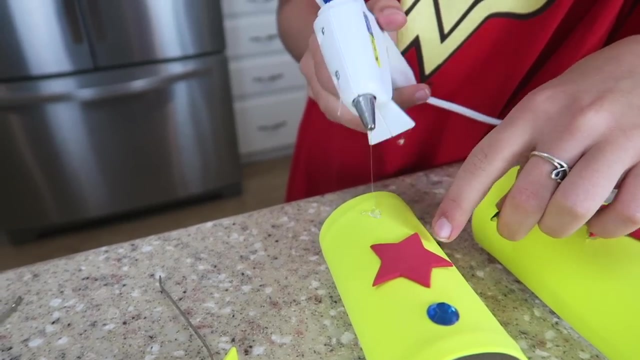 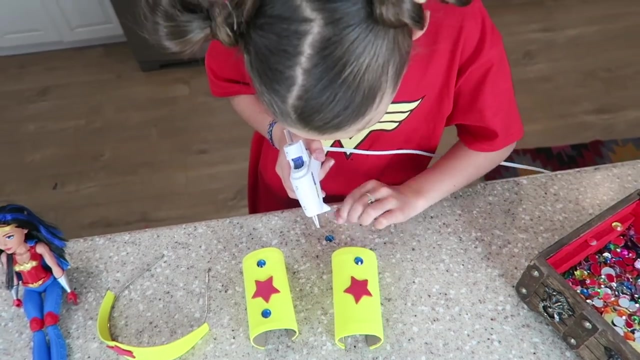 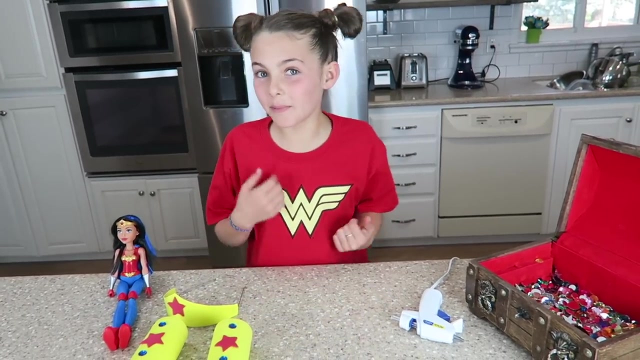 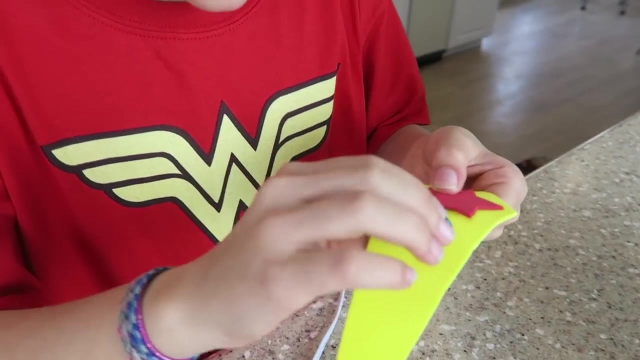 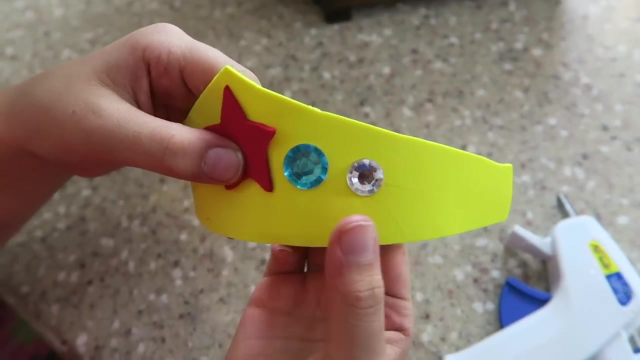 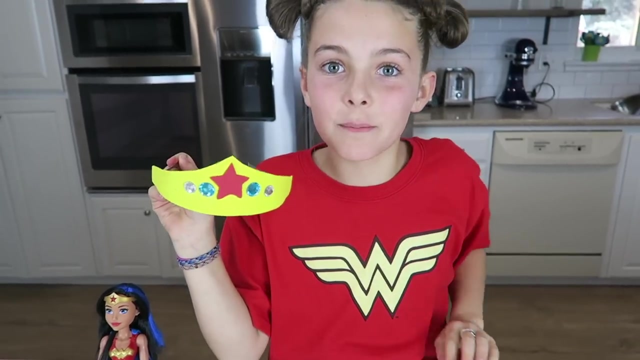 oh, I'm gonna add this blue gem, two blue gems, keep on dropping it. okay, there we go. all right, and I'm gonna put them right there now let's add some bling to that band. all right, big blue one, right there. there we go, ta-da. now let's put it all together and see what it looks like. 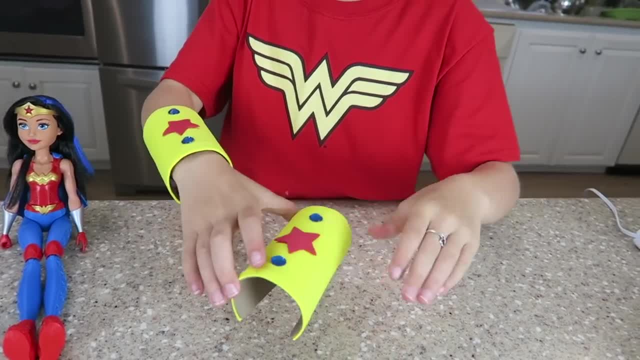 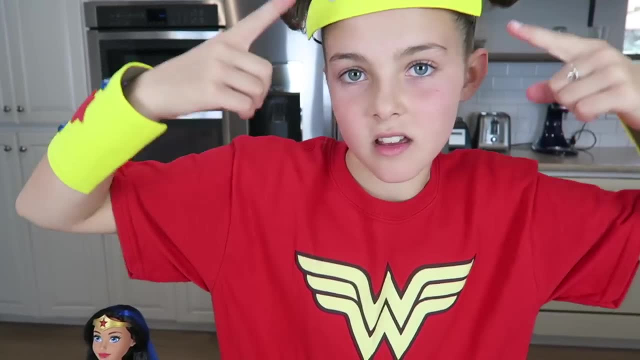 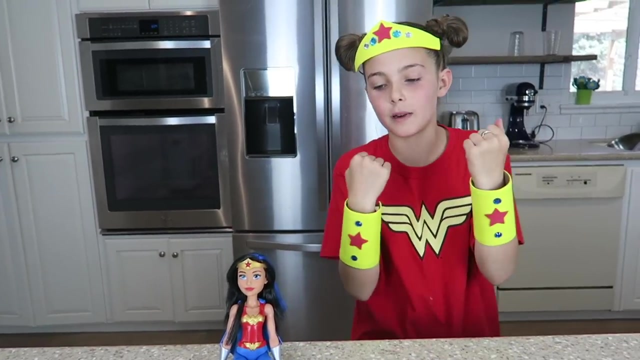 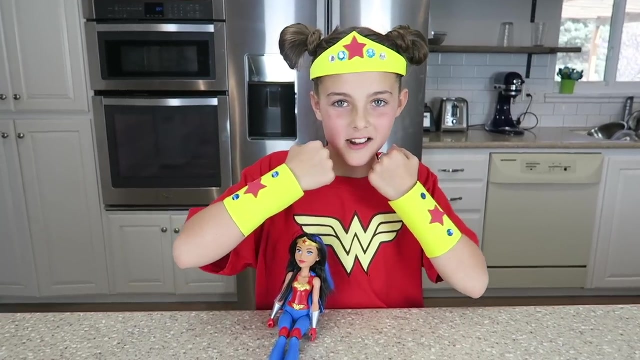 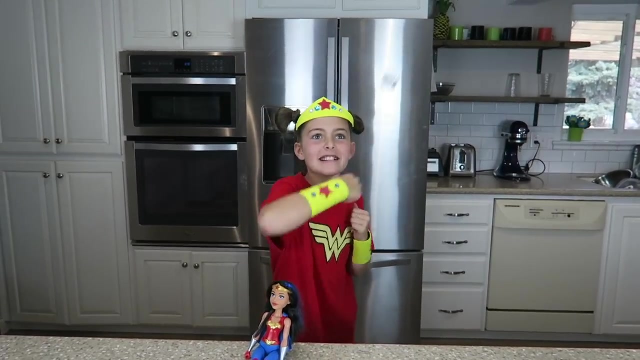 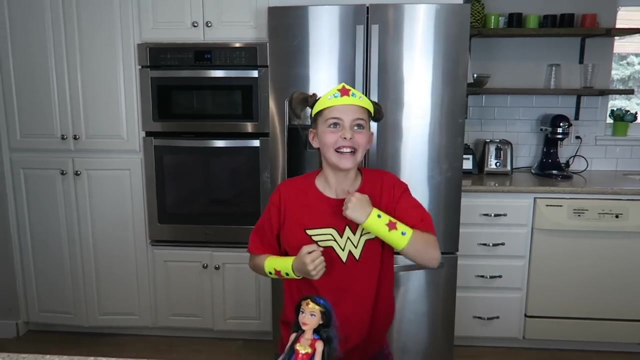 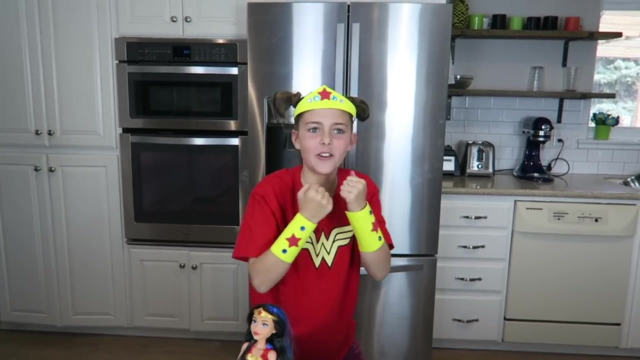 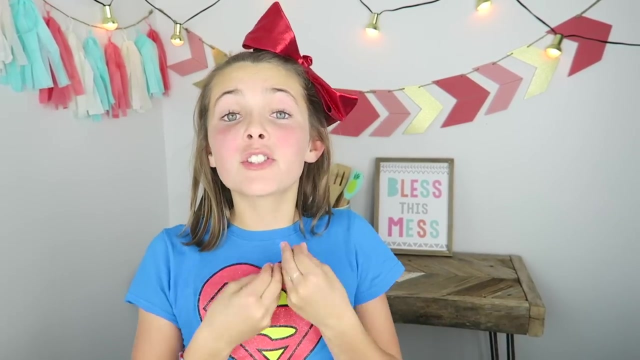 you, you, you. what do you guys think? pretty awesome, right? I like totally feel like a superhero. Wonder Woman. we're like twinners. should we see how good the bulletproof cups work? bring it on bad guys. yeah, yeah, I made it. I hope these ideas helped you out this year and hope you guys have so much fun.